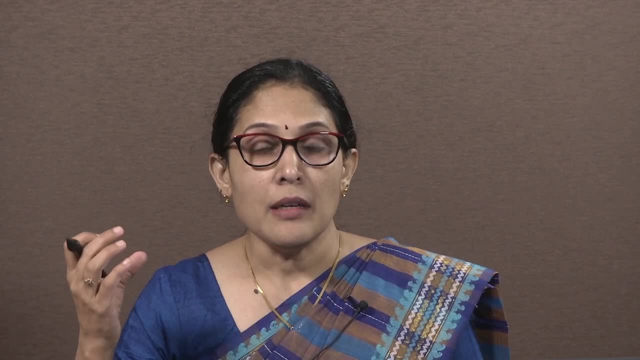 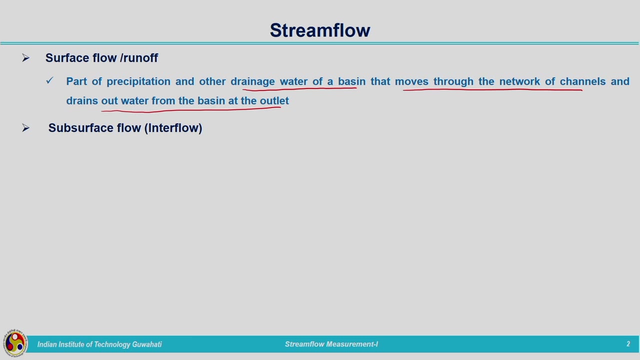 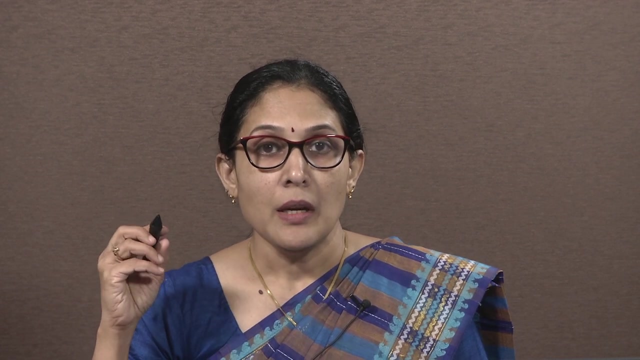 drainage water will be forming the runoff at the outlet of the watershed. Second one is subsurface flow or inter flow. What is subsurface flow or inter flow? We have already seen when we were discussing about subsurface water. In the case of subsurface, 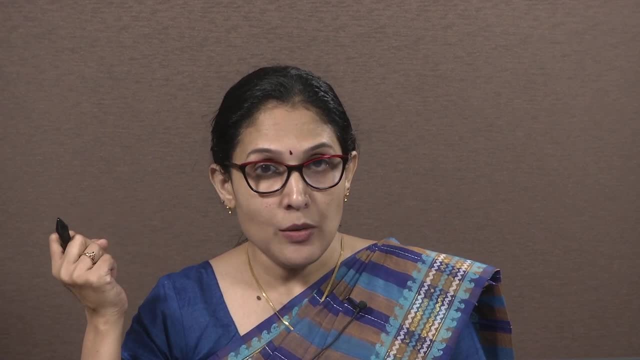 flow. what is happening, actually? Whenever precipitation is occurring, some amount of water is lost. When some amount of water is generated, some amount of water is transferred to the. whenever precipitation is occurring, some amount of water will be infiltrating into the soil. and the subsurface storage will be satisfied. After that the water starts flowing, depending on the gradient, So it will be flowing in the lateral direction and finally contributing to the streams. That is what is termed as the interflow, So the part of precipitation which infiltrate. 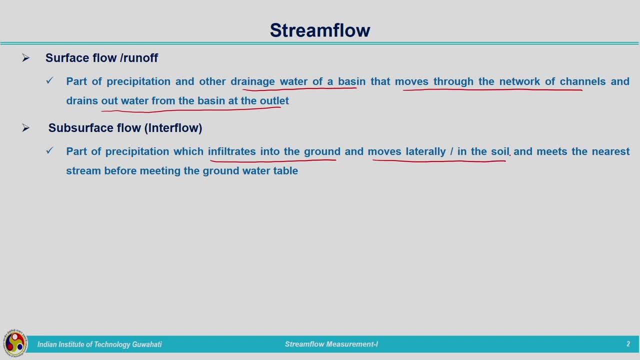 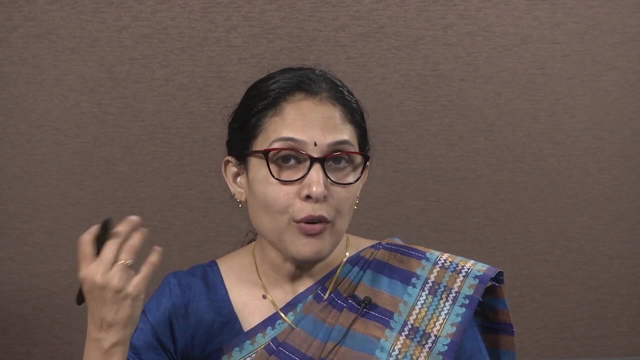 into the ground and moves laterally in the soil and finally meets the nearest stream before meeting the groundwater table. This water is not again moving downward to meet the groundwater table. Before that itself, it is moving laterally based on the gradient and finally contributing to 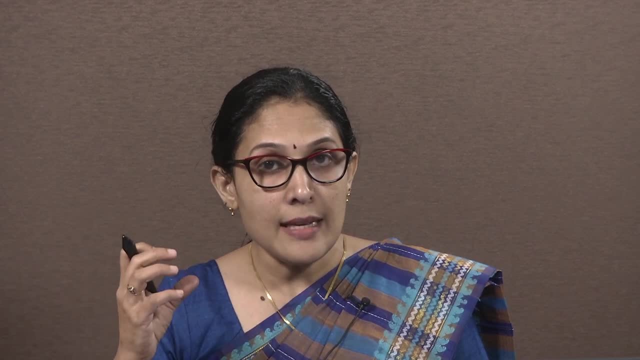 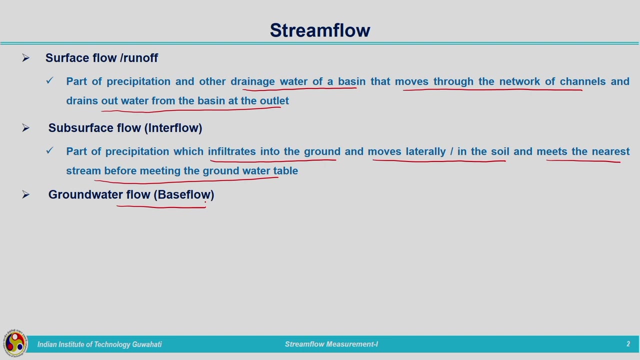 the stream, That is, the contribution from the unsaturated zone, is termed as the interflow. Next one is the groundwater flow or base flow. This is the contribution to the stream coming from the groundwater. Some amount of water will be available in the stream from the depletion. 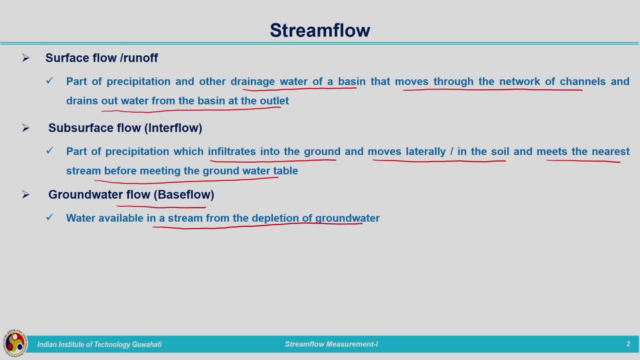 of groundwater, So this is termed as base flow. So when we talk about stream flow or total runoff of the basin, all these three components, along with the precipitation, comes into account. That is, flow, subsurface flow, groundwater flow and precipitation directly falling on the stream. 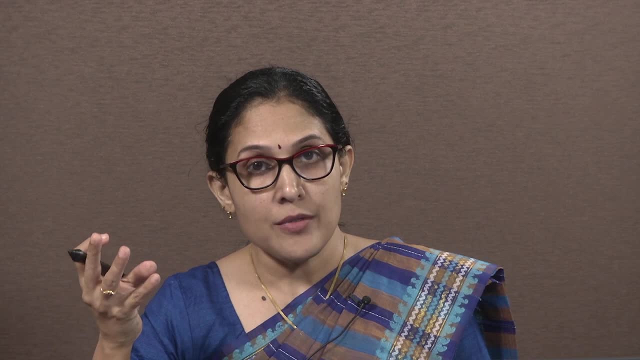 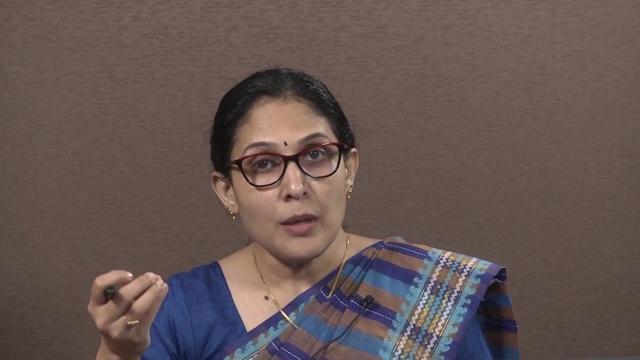 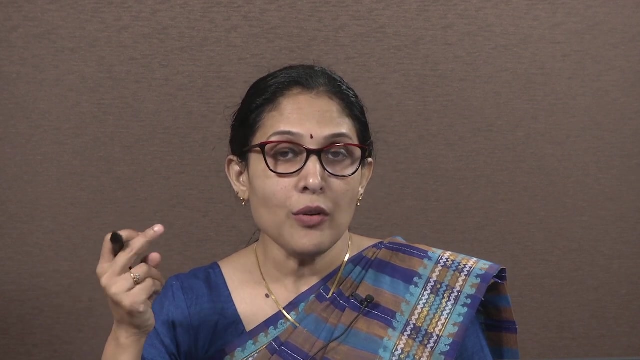 So the stream flow is consisting of the runoff, subsurface flow, That is the interflow, and groundwater flow, That is the base flow, and also the precipitation which is directly falling on the channel. together is termed as the stream flow. So the runoff for the surface flow is coming from the excess rainfall and the water which 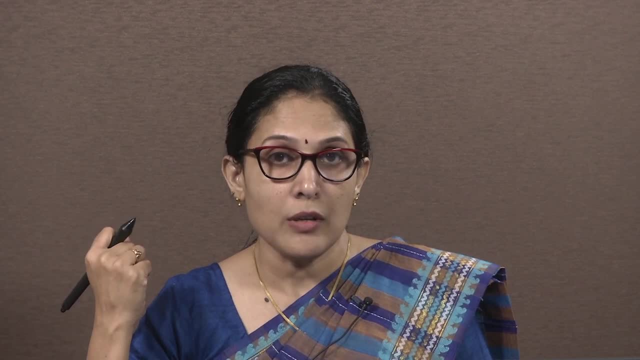 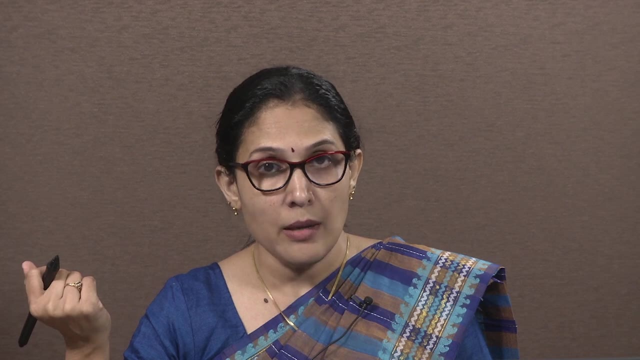 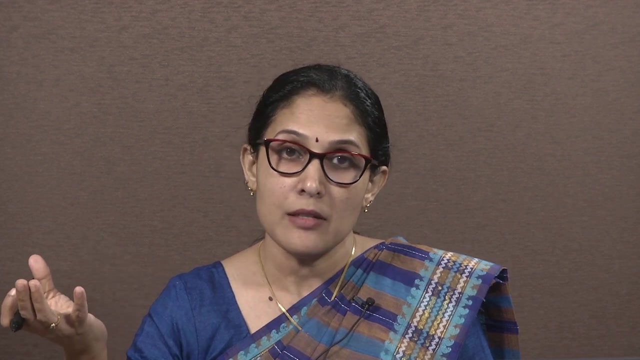 is coming, as interflow is based on the infiltrated water and again it is percolating to meet the groundwater table. that will be contributing towards the base flow. And in addition to that, rainfall is occurring on the watershed. it falls on the channels also. All these four. 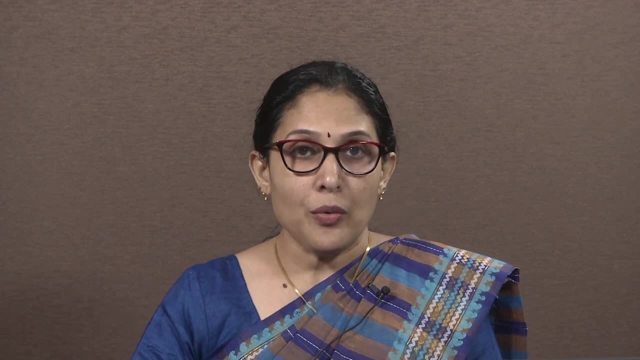 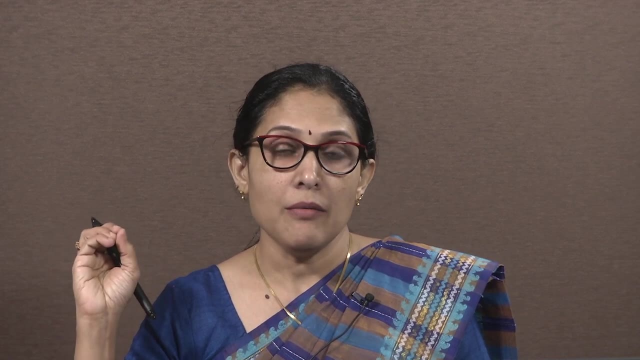 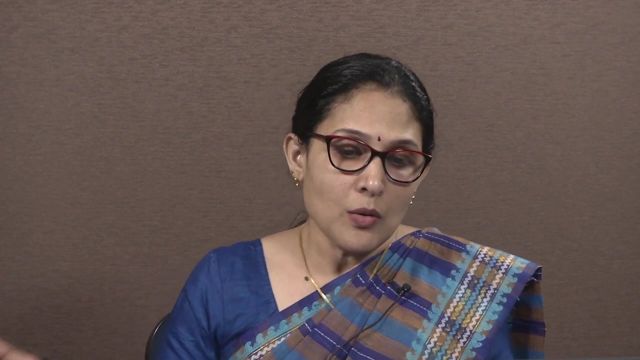 components, together termed as stream flow. So now we need to have mechanism for measurement of stream flow, because the stream flow is very important Whenever we are talking about any implementation of water resources projects. so it is measured in terms of units of discharge. What is the unit of discharge? It is in meter cube. 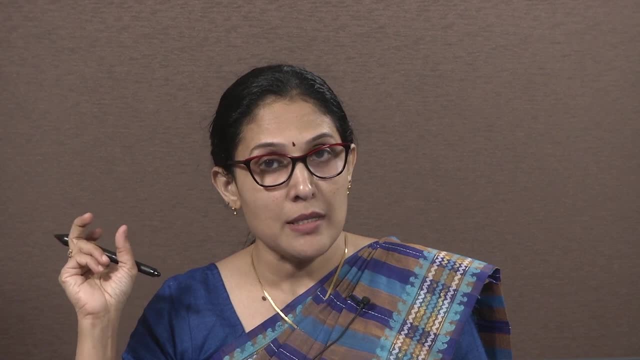 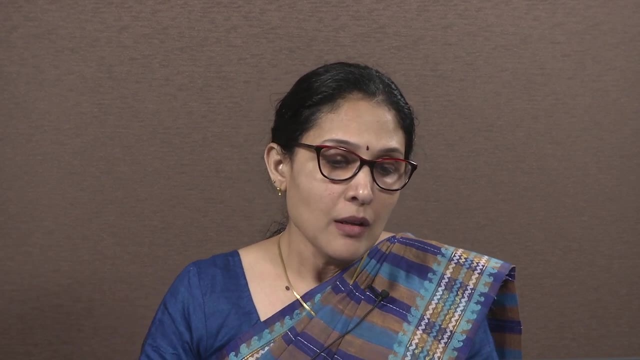 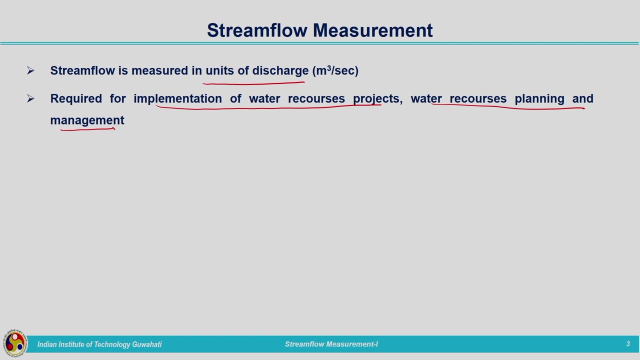 per second. Discharge is expressed in terms of meter cube per second. Same unit is used for representing stream flow also. So this is very important for the implementation of water resources projects, water resources planning and management, because whenever we are talking about the construction of a hydraulic 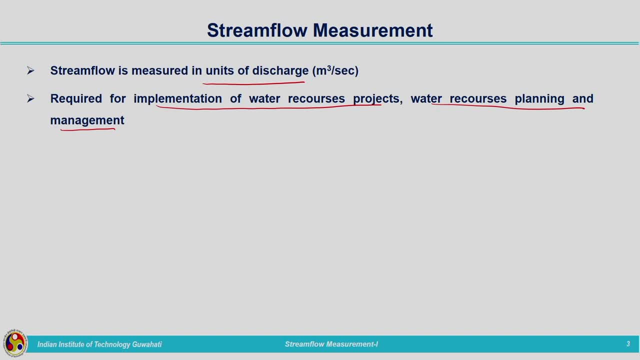 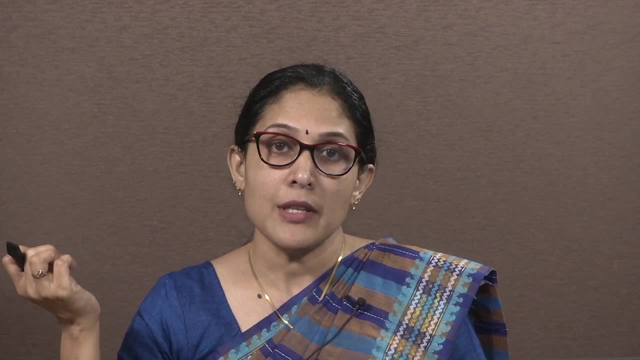 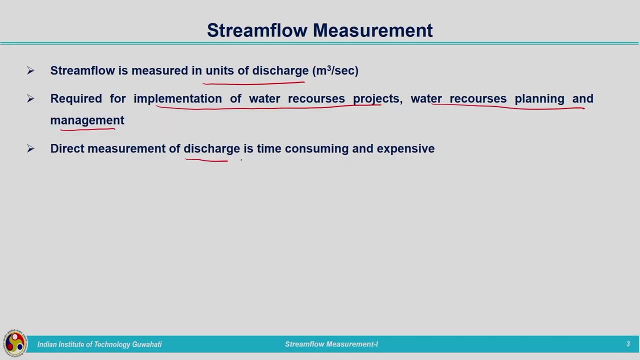 structure. we need to have the quantification of stream flow If we are going to provide some river protection, bank protection measures. in all these cases we need to have the idea about the stream flow which is occurring at that particular location. So direct measurement of discharge. 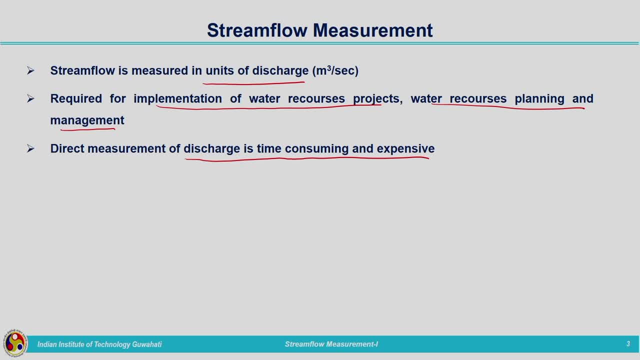 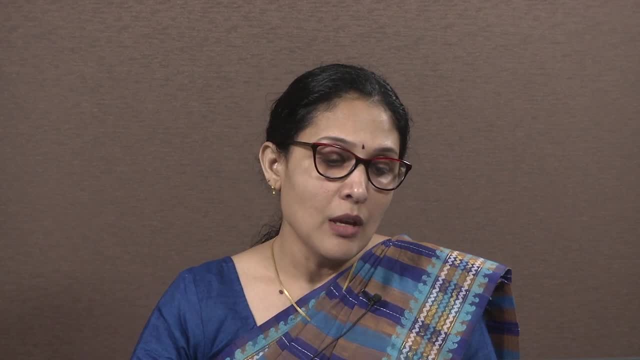 or stream flow, is time consuming and expensive, Even though we need to have the stream flow. the direct measurement is always very difficult and also time consuming. So what we will be going for? We will be going for indirect measurement of stream flow. How can it be done? It can. 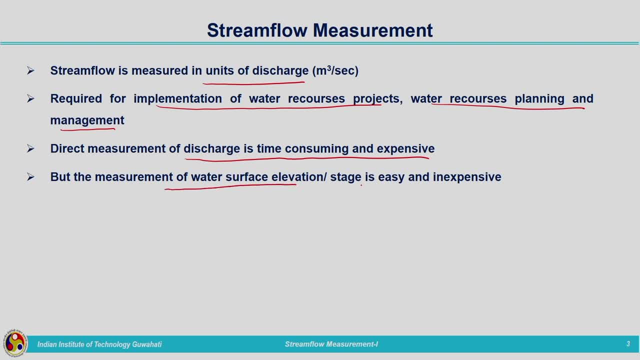 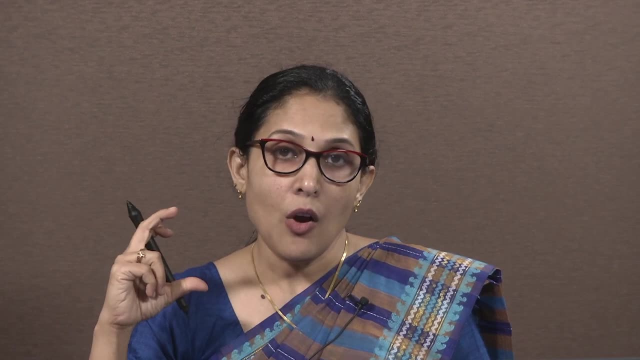 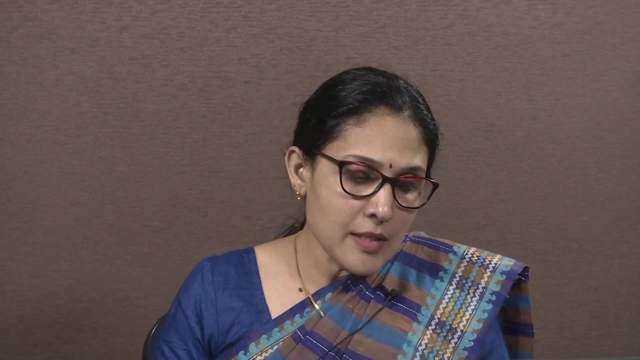 be done by the measurement of water surface elevation. that is less time consuming and inexpensive. Water surface elevation is also termed as stage. Stage measurement means water surface elevation, determination of water surface elevation. How much is the water depth prevailing in the particular stream? That is termed as stage Stage is nothing but the. 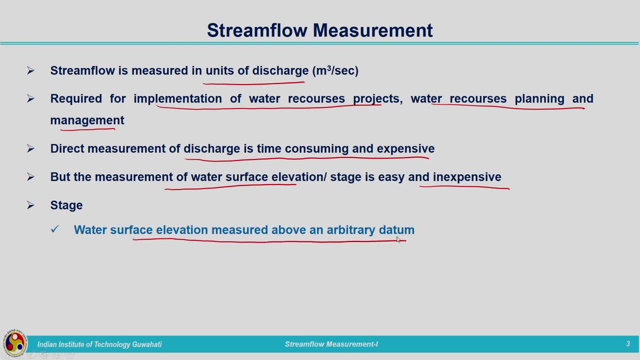 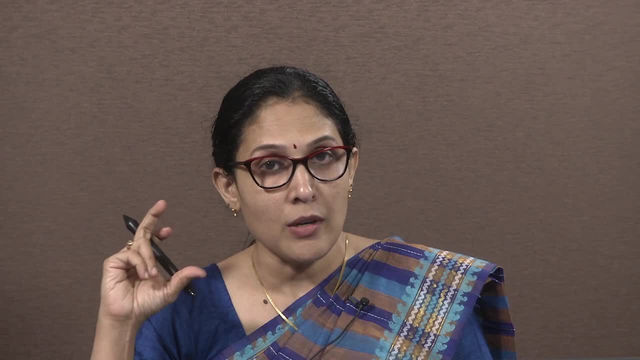 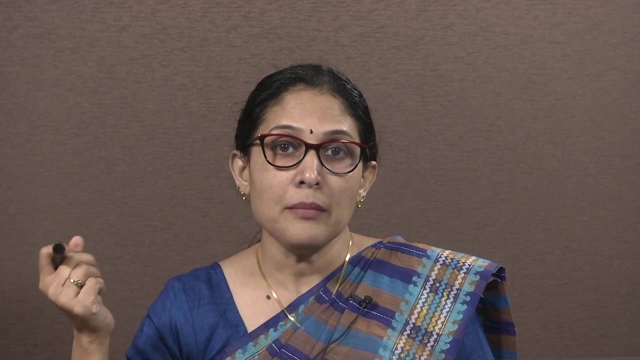 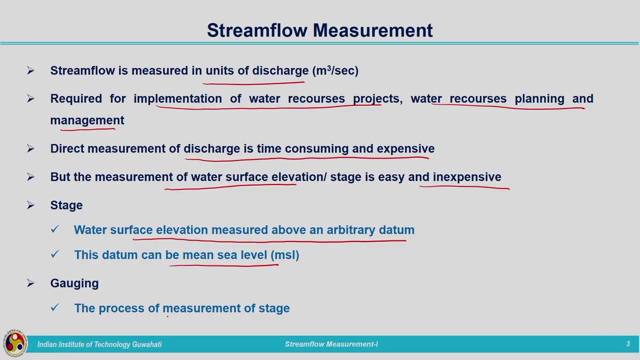 water surface elevation measured above an arbitrary datum, and this datum can be mean sea level. We need to have a datum based on that we will be measuring the water surface or water level. Water surface elevation is measured based on the datum That datum them. usually we consider as the mean sea level And this process of measurement of stage is 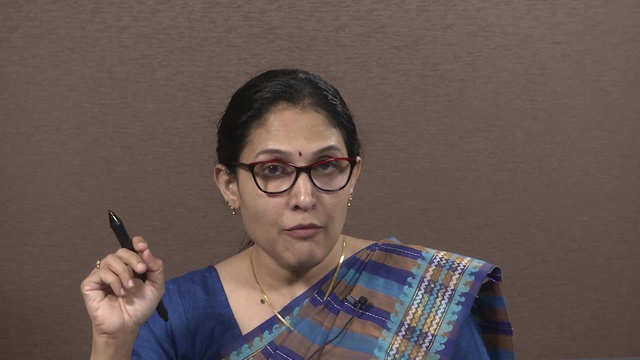 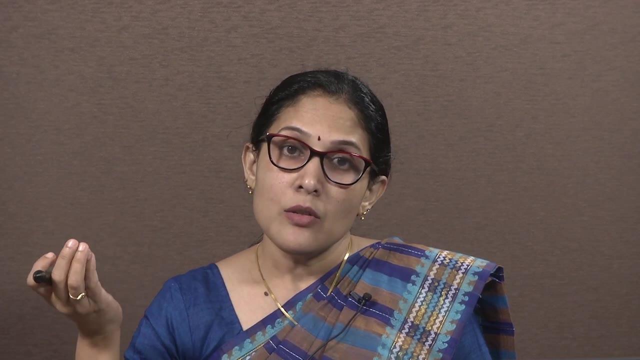 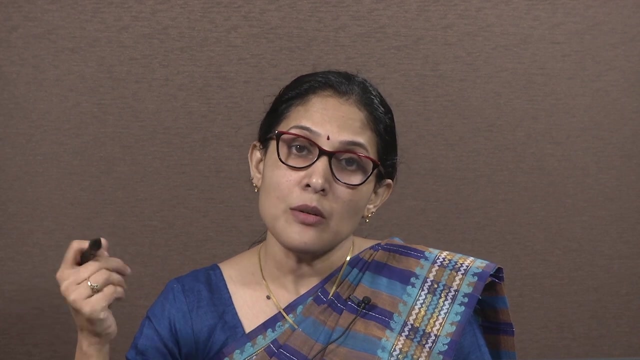 termed as gauging. So when we talk about stream flow measurement, measurement of this stream flow is a difficult process and also time consuming, So we will be always going for indirect measurement of stream flow by measuring the velocity and also water level. 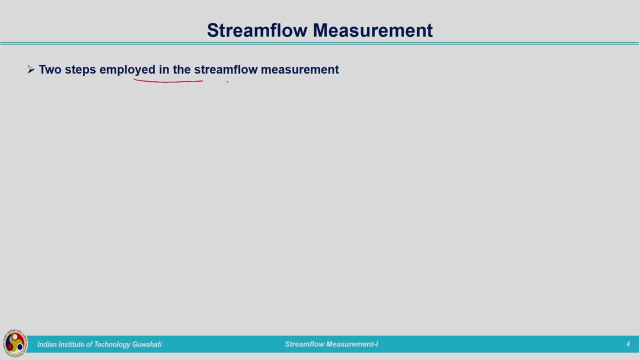 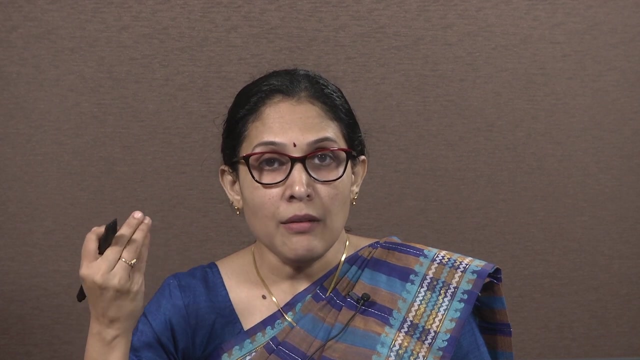 measurement. There are two steps involved in the stream flow measurement: step 1 and step 2.. In step 1, discharge of the stream is related to the stage. using series of measurement. We will be measuring the stage at a particular station, gauging station and corresponding 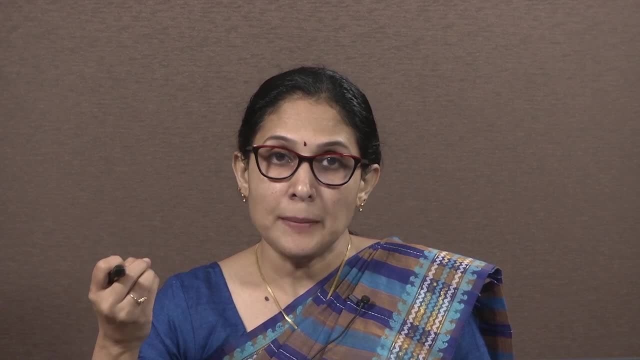 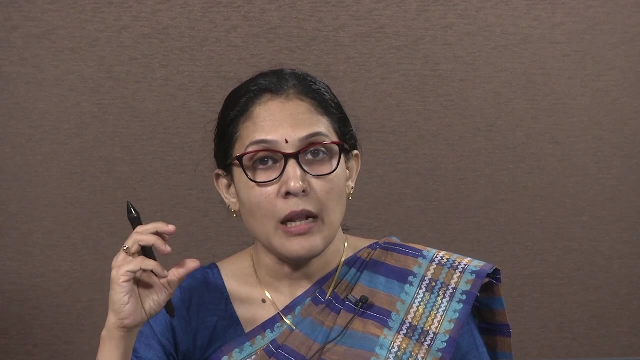 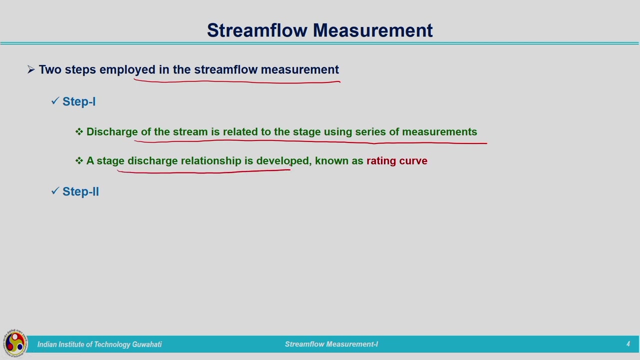 velocity at that particular gauging station measured. Base on the stage and width of the river and also the velocity measured, we can calculate the discharge at that particular gauging station. After that, a stage discharge relationship is developed, which is known as well known rating curve. This rating curve is very important. 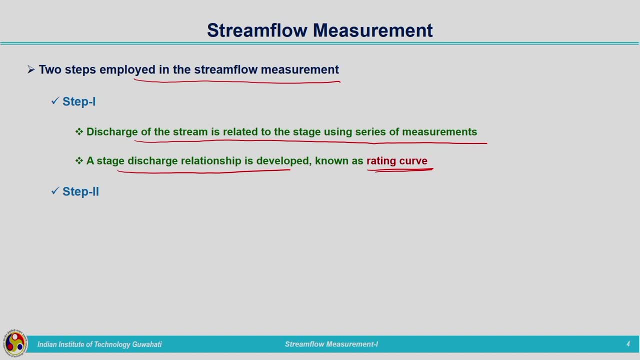 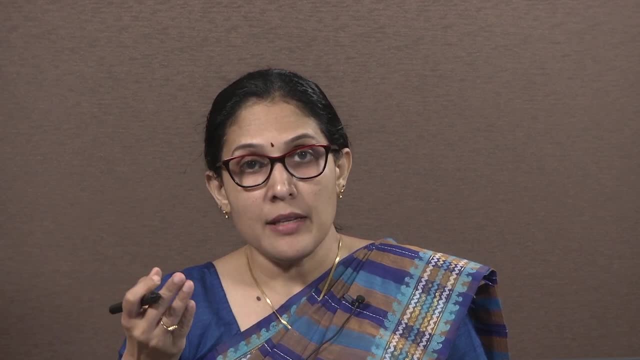 How this rating curve is formed. We will be plotting the data corresponding to water level and the corresponding discharge. So for a particular gauging station, we will be calculating the direct flow rate in the depth of the strait surface of the water mixture, which means 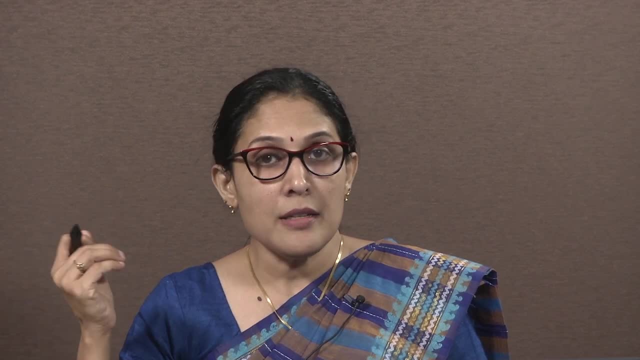 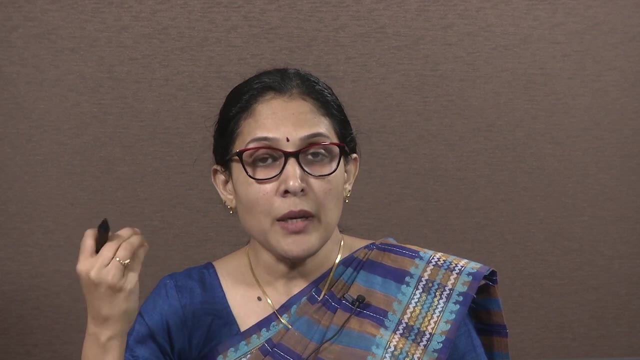 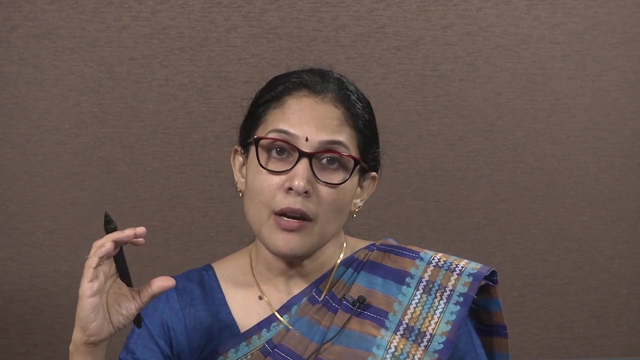 we will get the average flow rate, this length mile pressure challenge level, which will be applied for theè critical water level threshold, So 2.4 unit Id per meter square water level, which is defined as the dose of discharge that can be given by the. 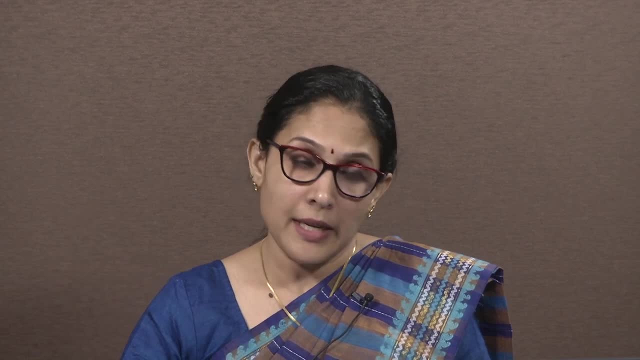 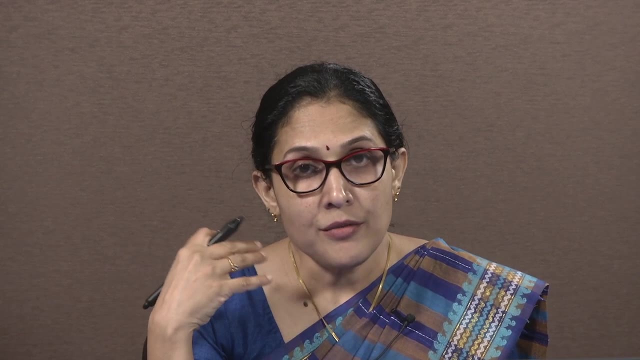 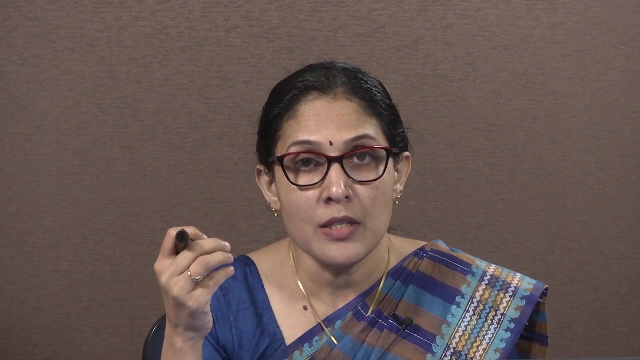 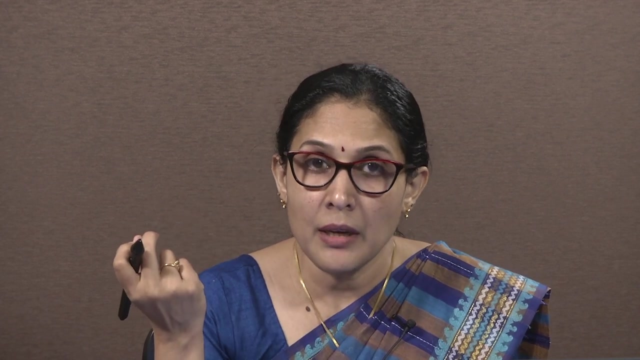 of stage discharge rating curve will be done Then in step 2, after formulating the rating curve, after certain time period, maybe in different season, we will be measuring the water level or stage and, corresponding to that stage, what will be the discharge that will be noted from the 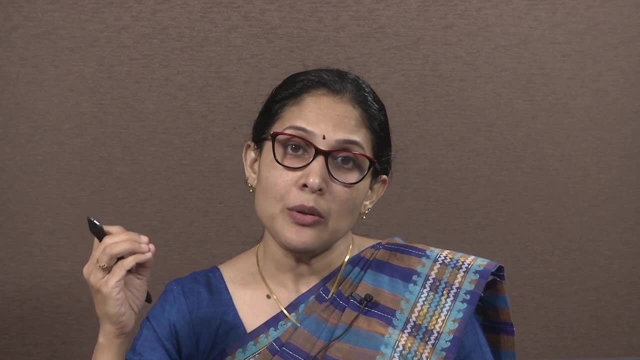 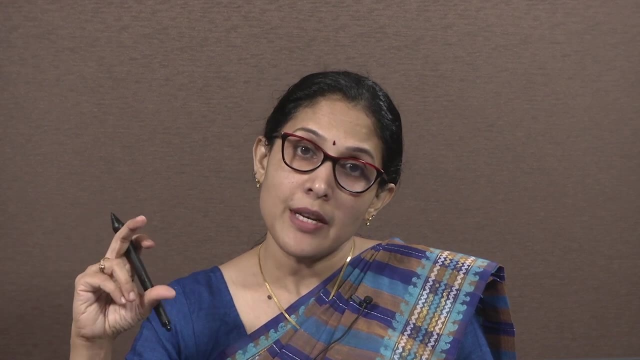 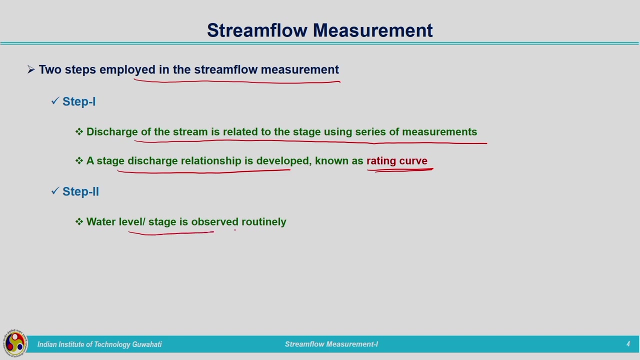 rating curve. So every time there is no need to go for measurement of discharge, that is measurement of stage and velocity. only stage is required if rating curve is already formed for a particular gauging station. So second step, what we are doing, water level or stage is observed. 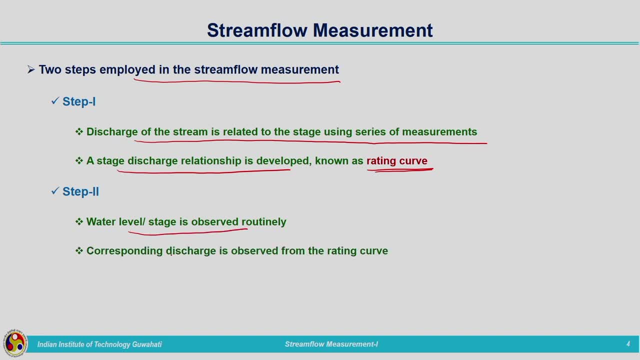 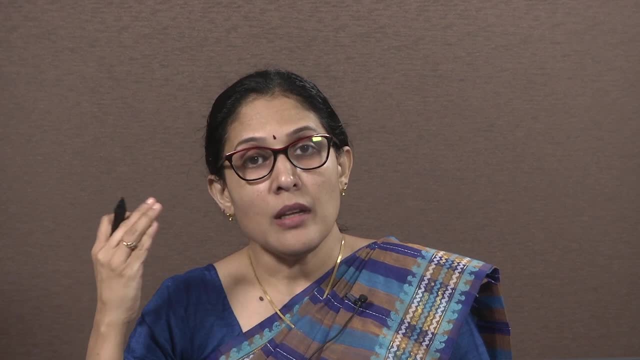 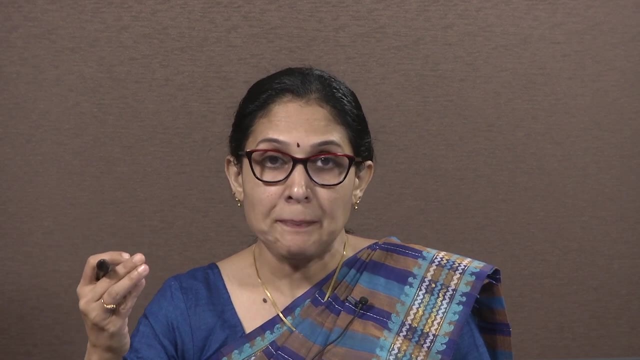 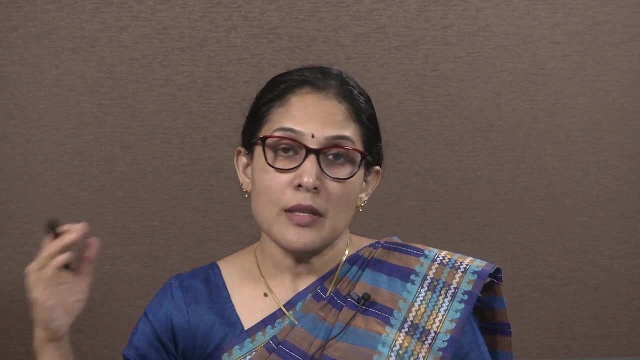 routinely and corresponding discharge is observed from the rating curve. The water level observation is done routinely by certain agencies. So always, discharge measurement won't be done. water level measurement will be done and corresponding to that water level we can get the discharge from the rating curve. So this is the 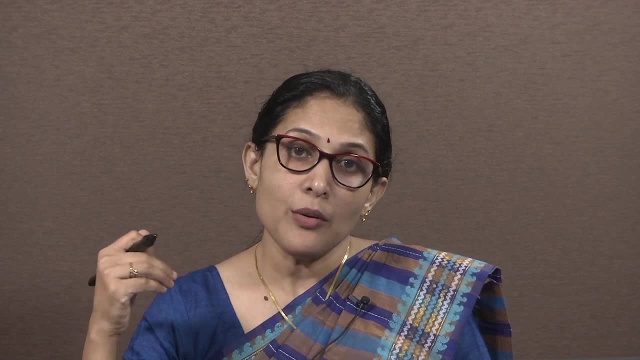 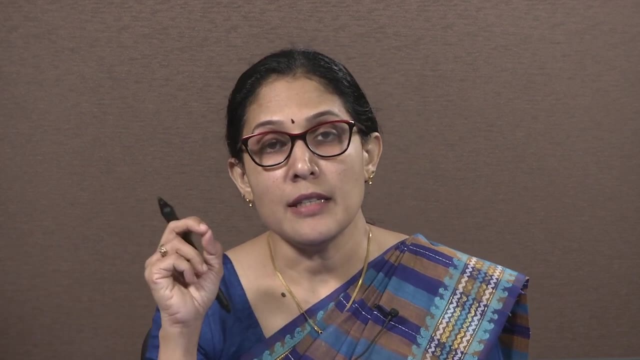 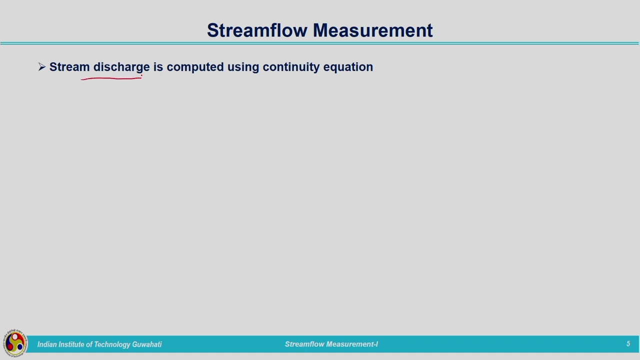 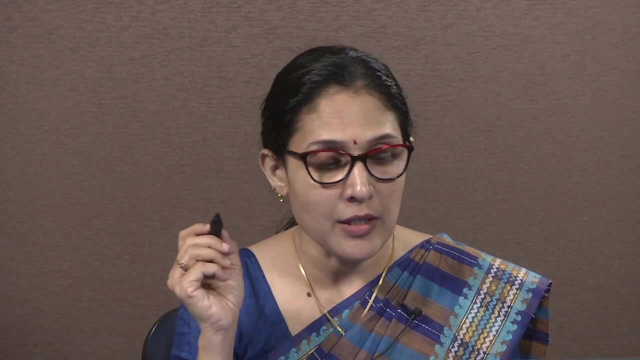 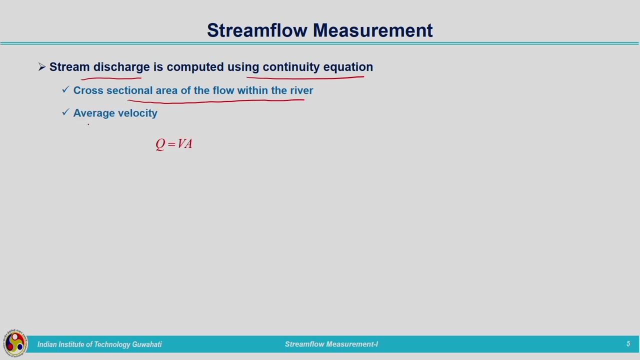 way, which we look forward, to get the stream flow in a particular gauging station rather than directly measuring the stream flow. So, after getting the stage at a particular location, how can we determine the residual flow? or� do we object to these experiment? airplanes are actually brightly emitting low and low". 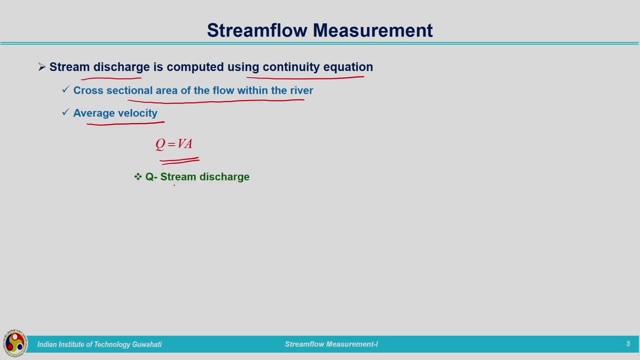 Yeah, high and low, Beweg mogę åtКive Earth. if�� Q is equal to VA, Q is the stream discharge, V is the average velocity, A is the cross-sectional area of the flow within the river. Now let us move on to the topic of determining. 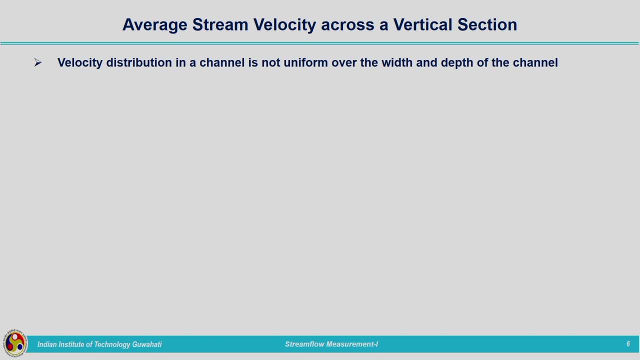 average velocity, average stream velocity, That is, average stream velocity across a vertical section. We all know velocity distribution in a channel is not uniform over the width and depth of the channel. When we talk about the velocity distribution in a channel or in a river, 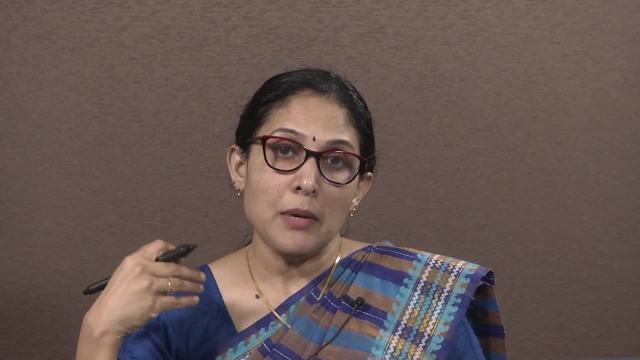 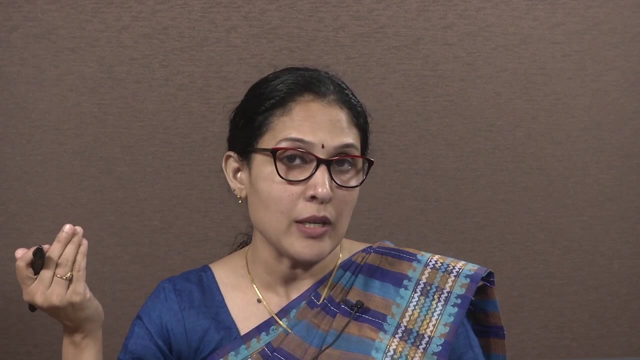 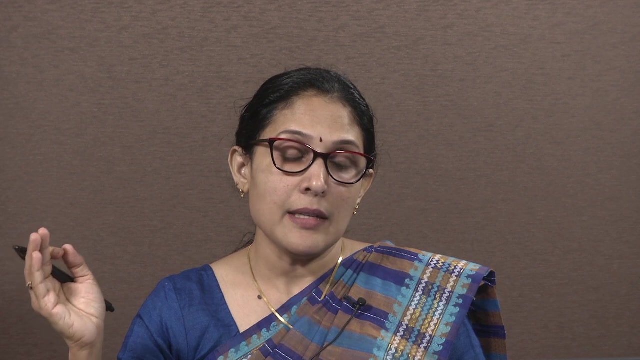 it is not uniform. For simplification purpose, we used to consider the flow to be uniform and uniform velocity will be calculated by using the corresponding formula. But always it is not like that In actual condition. it is not uniform across the width and also depth. 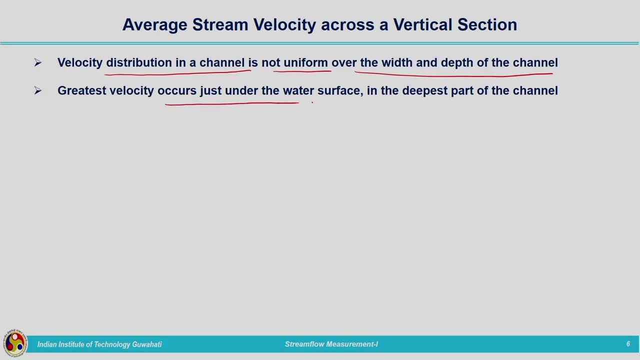 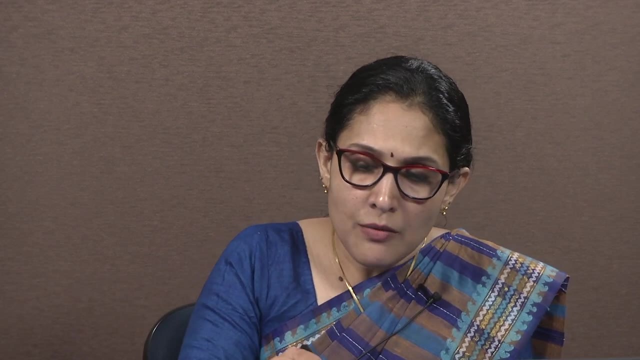 The greatest velocity occurs just under the water surface. in the deepest part of the channel. It is not on the water surface. Certain depth below the water surface the maximum velocity will be occurring. Velocity distribution across a vertical section is approximately logarithmic in nature. 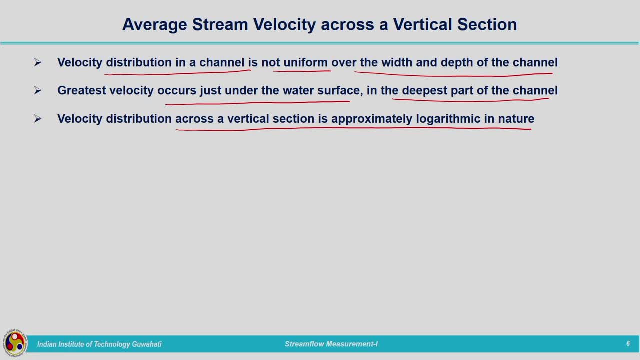 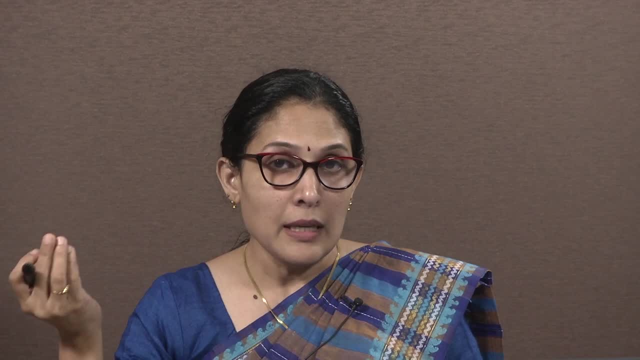 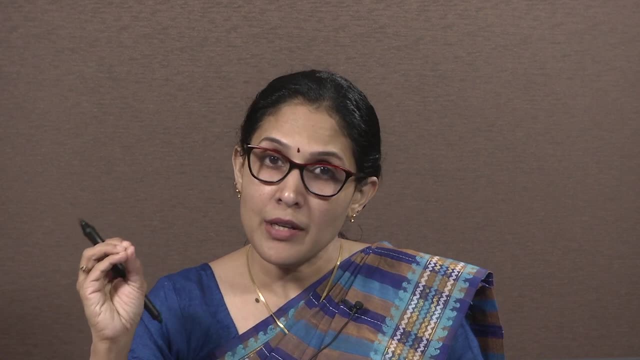 When we plot the velocity distribution curve it is logarithmic in nature. I am not going deep into those details how the velocity distribution will be in an open channel. that you might have covered already in open channel hydraulics. So here what we want: we want the average velocity. 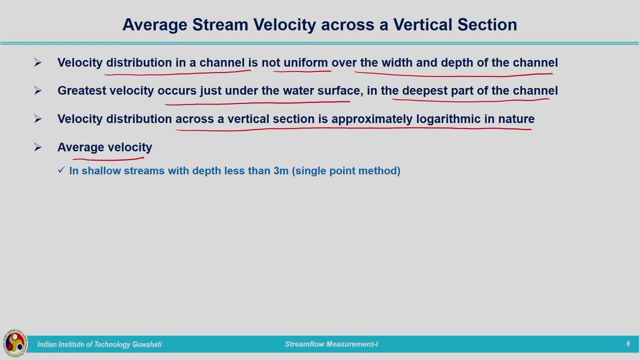 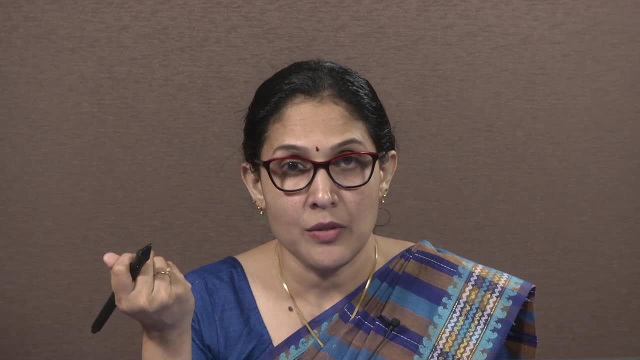 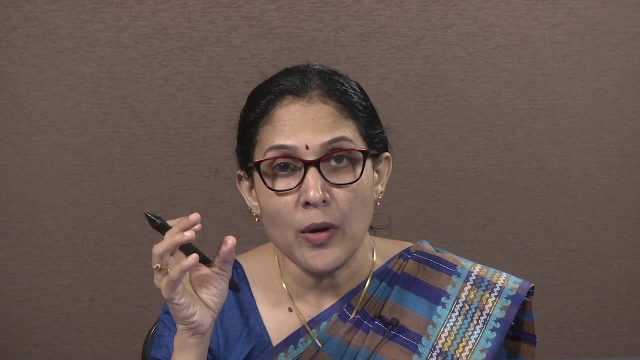 For that what we are doing. we will be measuring the velocity at different depths And based on the velocity measurement we will be calculating the average velocity. There are different ways to get the average velocity. Commonly will be using 1-point method and 2-point method, So in shallow streams. 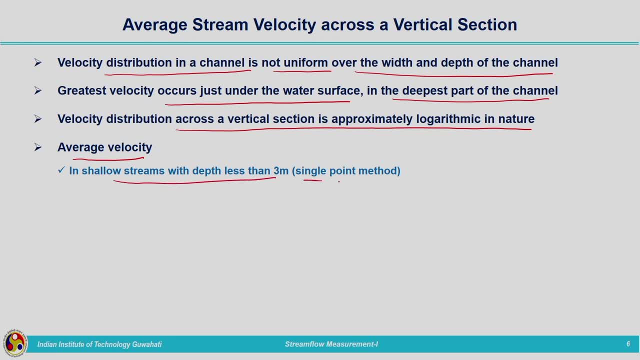 with depth less than 3-meters will be using single-point method. What is meant by the single-point method In this? what we are doing? we are measuring the velocity at a depth of 0.6 times the depth of the stream. We know the water depth. Water depth will be measured. 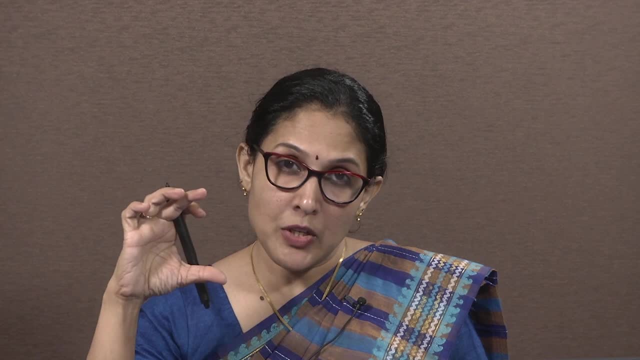 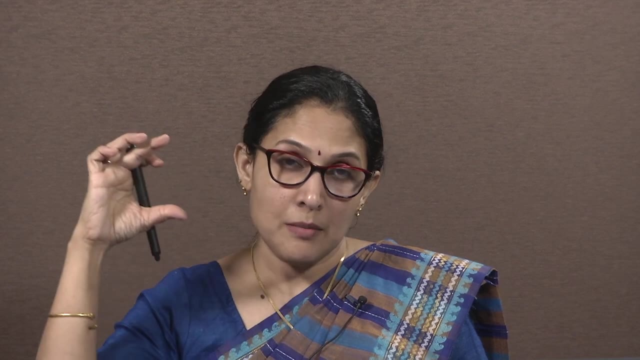 But also we are not going to be using single point method In this. we are not going to measure the water depth, Weratospan ____�. we start by measuring the velocity at a depthны be measured. Based on that, we will be determining the position where the depth is 0.6 times the. 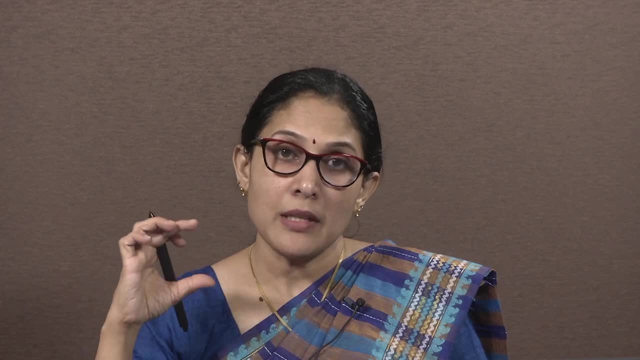 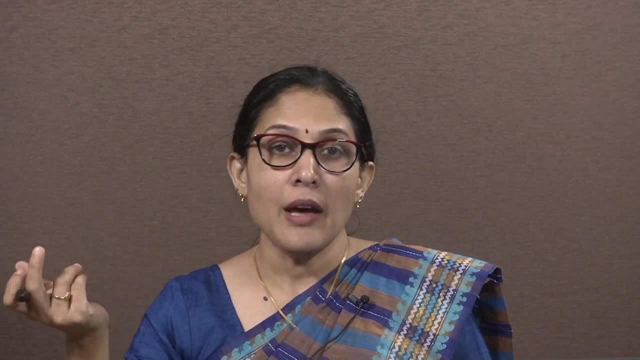 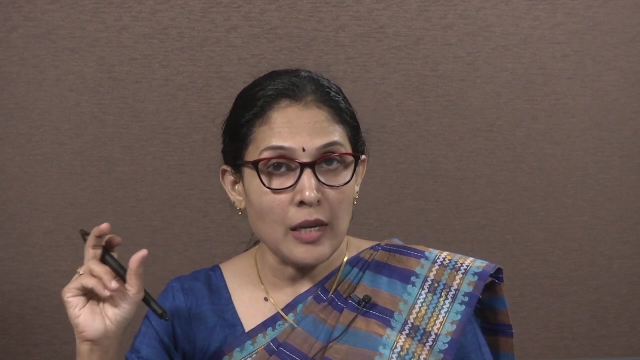 depth of the channel. At that location, we will be measuring the velocity. We will be measuring velocity at two different depths and we will be taking the average of those two values to get the average velocity. This is an approximate way, approximate method to calculate. 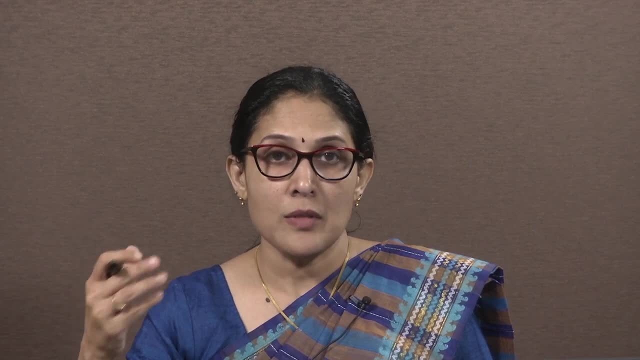 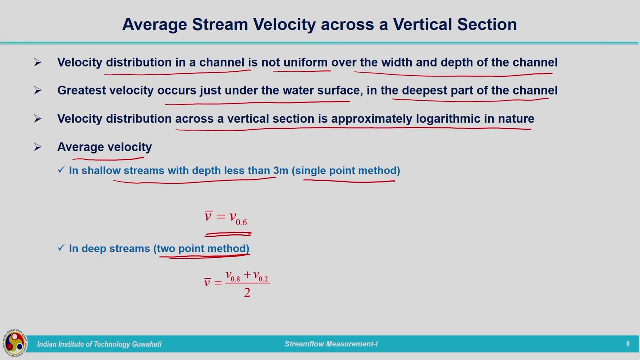 the average velocity. Both these methods are approximations only and in deep streams what we are doing. average velocity is equal to V0.8 plus V0.2 divided by 2.. What are these V0.8 and V0.2?? 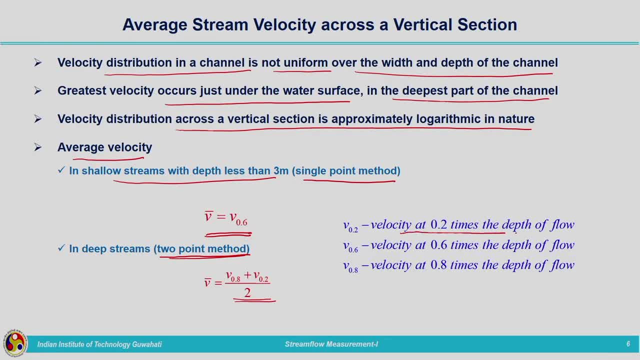 V0.2 is the velocity at 0.2 times the depth of flow, V0.6 that we have seen in the single point channel as V0.7 and V0.8. So V0.6 is dead. V0.0 remains when V0.8 is dead. 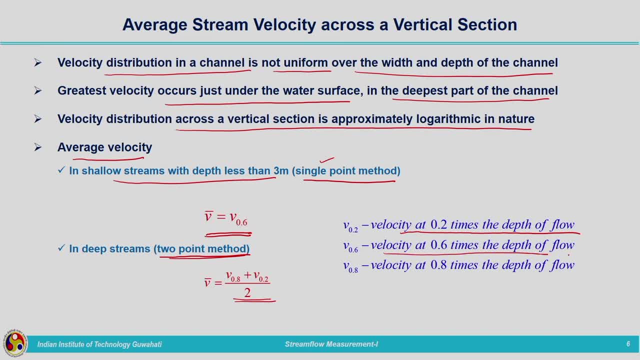 These are the wrong values for each one of these cameras. neighbourhoods can be themselves watching point. method is the velocity at 0.6 times the depth of flow and v 0.8 is the velocity at 0.8 times the depth of flow. So that way, in shallow streams, we will be measuring the 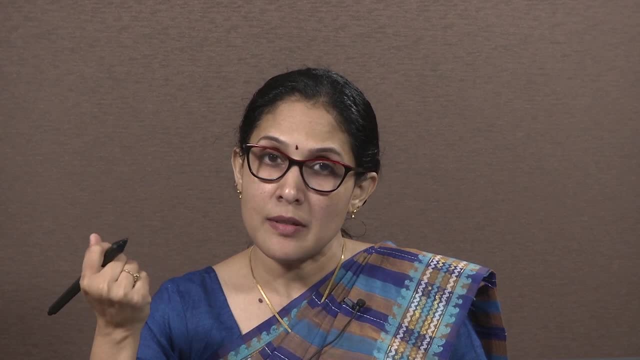 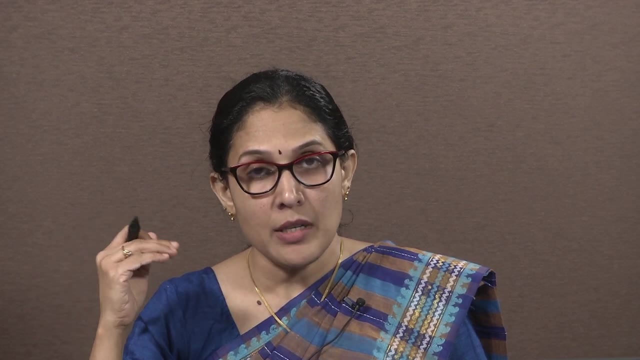 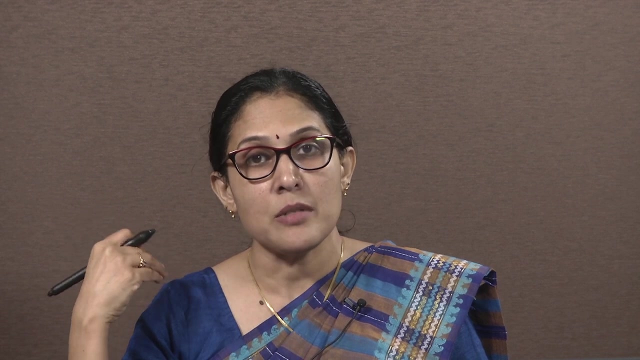 velocity at a single point, that is, velocity at 0.6 times the depth of the stream. And in the case of deeper streams, we will be measuring the velocity at 2 points, that is, at 0.2 times the depth of the stream and also 0.8 times the depth of the stream. the 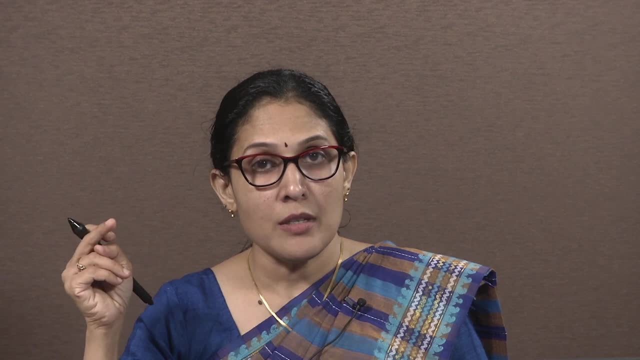 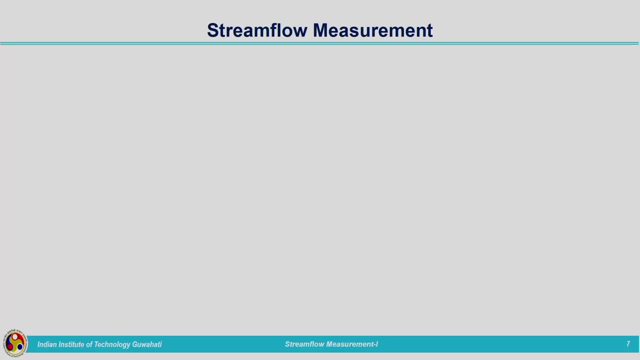 velocities will be measured. The average of these 2 velocities is considered as the average velocity of the stream. Now let us move on to stream flow measurement. that is, we need to have stage measurement techniques, we need to have velocity measurement techniques and after that we need to calculate the stream flow. 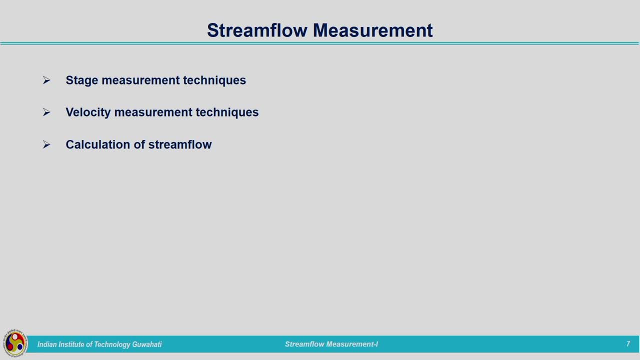 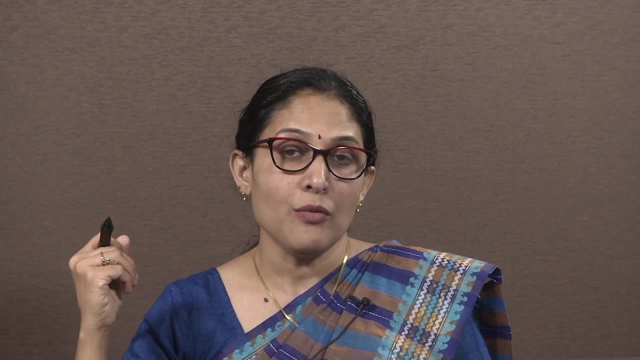 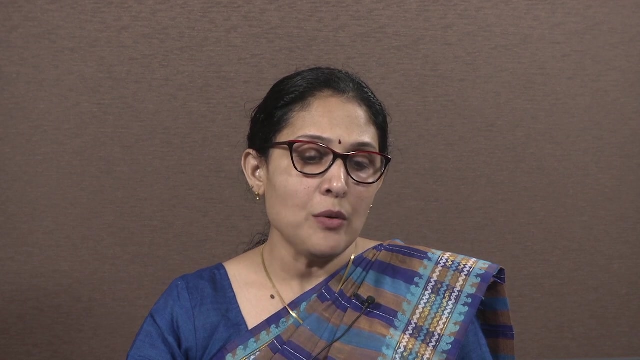 First we need to measure stage and velocity. Once the stage and velocity are measured, after that we can go for the calculation of stream flow. So in this lecture we are going to look into stage measurement techniques and velocity measurement techniques. in the next. 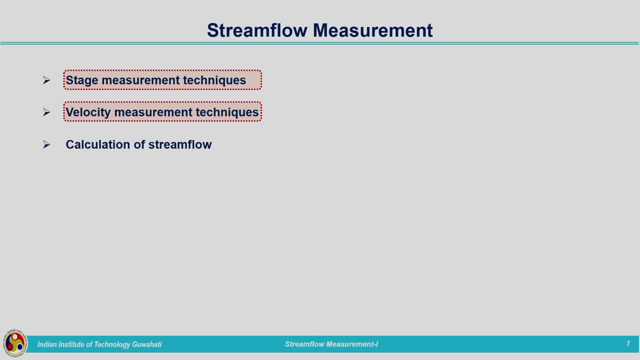 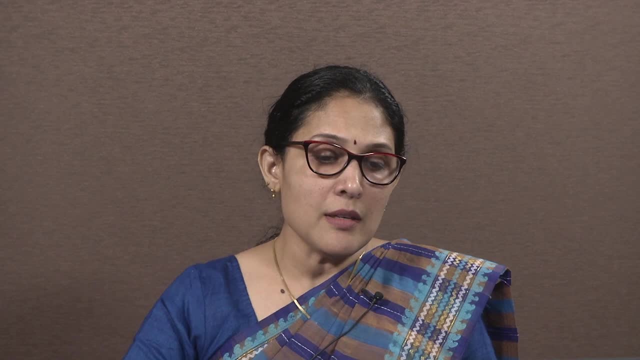 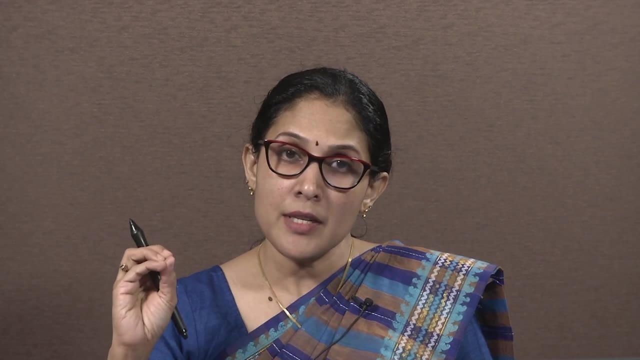 lecture we will move on to calculation of stream flow that we have already seen, that is, by making use of the continuity equation. q is equal to av. So let us start with the Stage measurement techniques. different measurement techniques are the which are very commonly used, or conventional techniques we will be looking into in this lecture. 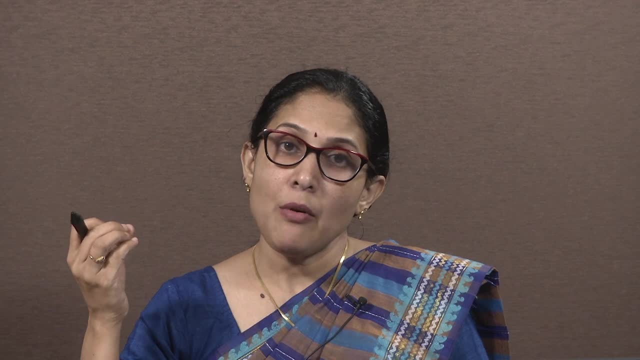 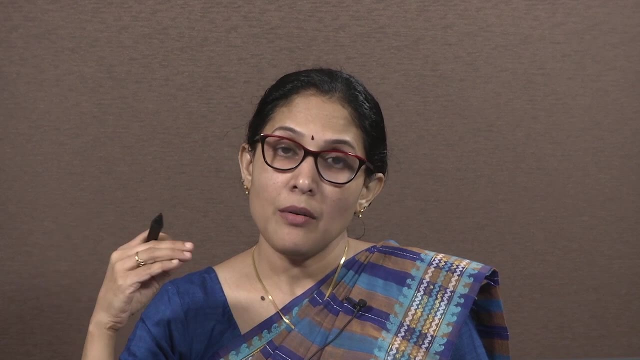 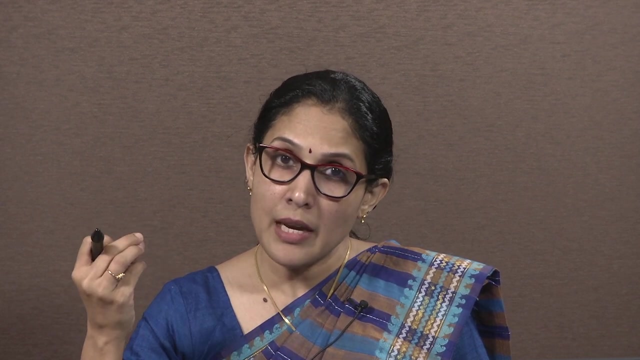 As we were talking about rainfall. when we were discussing about rainfall, we have seen two different techniques: are the recording type and non-recording type, that is, manual and automatic. In the similar way, in the case of stream flow also, we are having two different types. 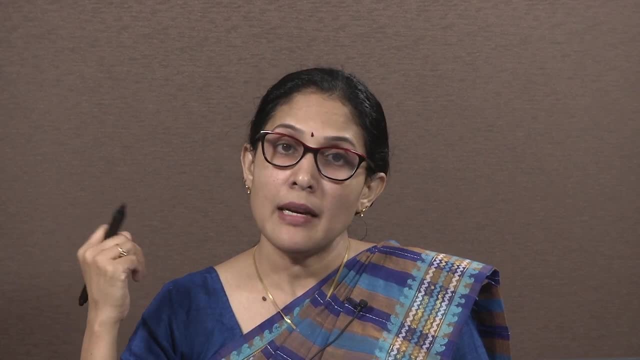 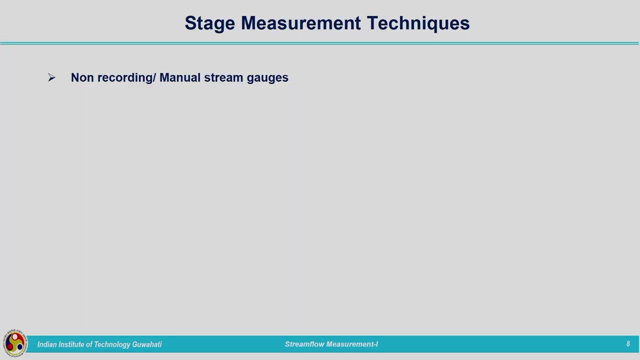 of measuring methodologies. one is recording and the other one is the non-recording. So let us see different stage measurement techniques: non-recording or manual stream gauges. that is, in that I am going to include staff gauge, wire gauge and electric tape. 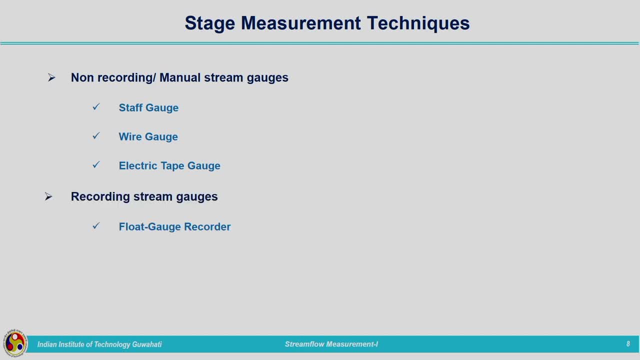 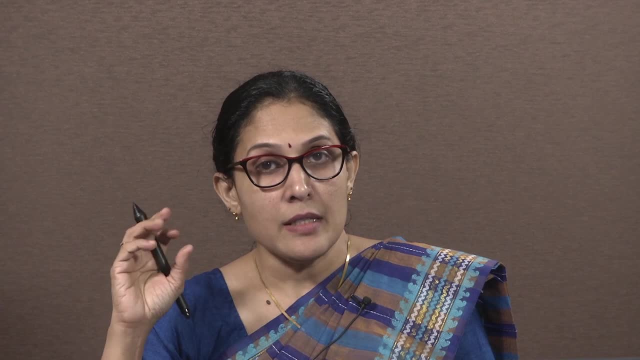 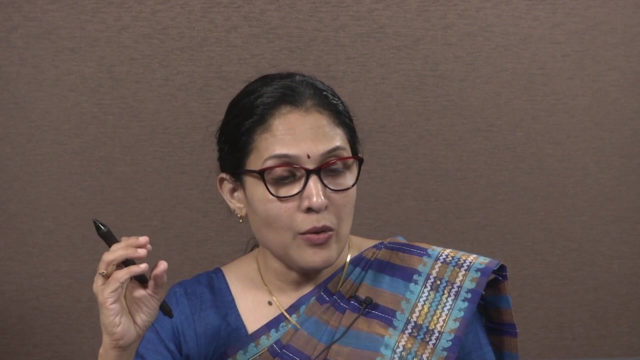 gauge And recording stream gauges. we will be looking into float gauge recorder. So regarding wire gauge stage measurement techniques, two types of methods are there. one is recording type and the other one is non-recording. under non-recording staff gauge, wire gauge and electric tape gauge will be seen. 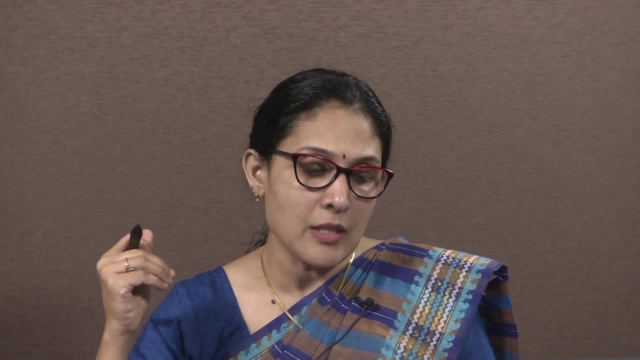 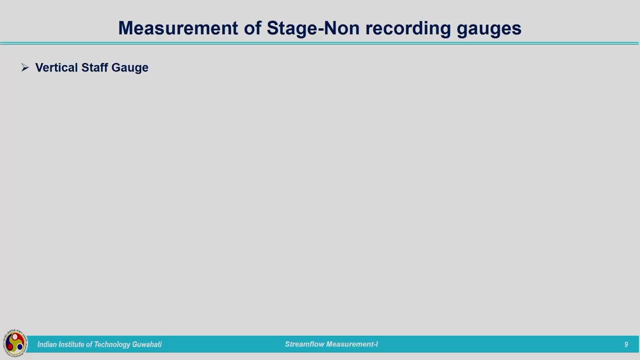 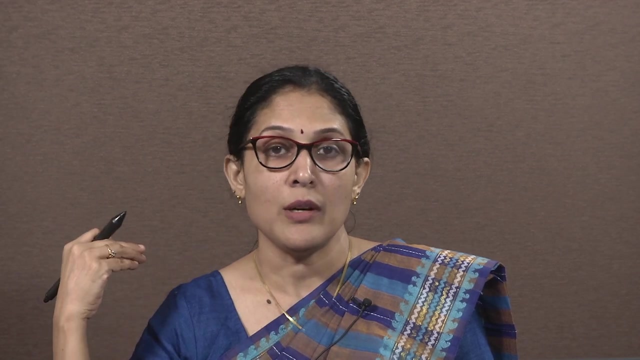 and in the case of recording stream gauges, we will be looking into float gauge recorder. let us see one by one. first one is the vertical staff gauge. vertical staff gauge why? specifically mentioning there are certain type of gauges in which inclined one also placed. so here let us see. 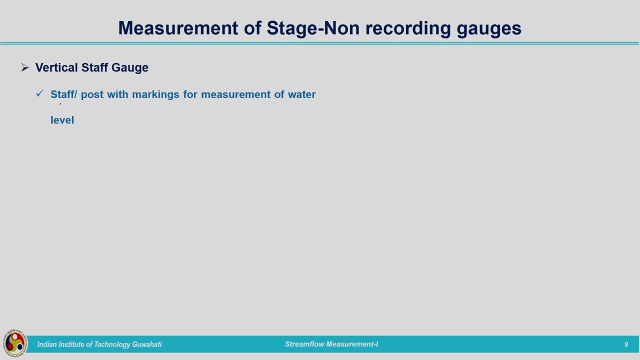 what is vertical staff gauge? this is nothing but a simple staff or post with some markings of the length for measurement of water level. so this one staff is there or a post is there. on that, the markings- length markings- are made based on the water level corresponding to that. 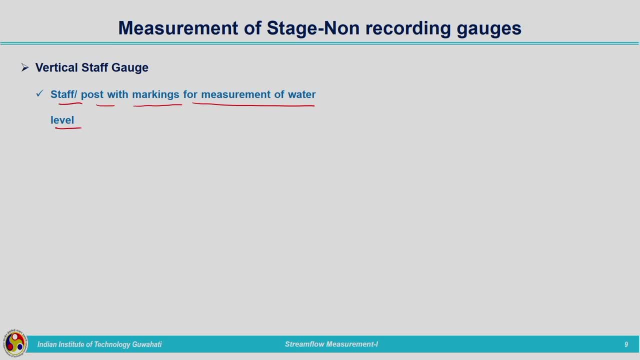 staff level line line. line line line can get the water level or stage at that particular location. how it is done, let us see this is fixed either to the abutment or pier or some wall. some hydraulic structure will be present in the stream. to the wall of that particular structure or pier it will be attached. this staff will be attached. 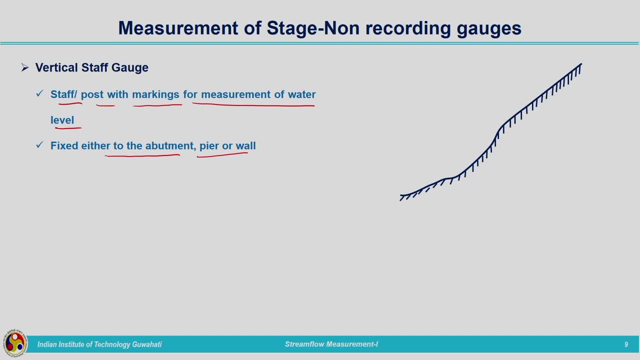 we can see it by means of a schematic diagram. this is the riverbed and water surface elevation is up to this, that marked by this blue line, and we are having the hydraulic structure bridge and this is representing the bridge deck slab and this is our abutment. this is the abutment of the bridge. 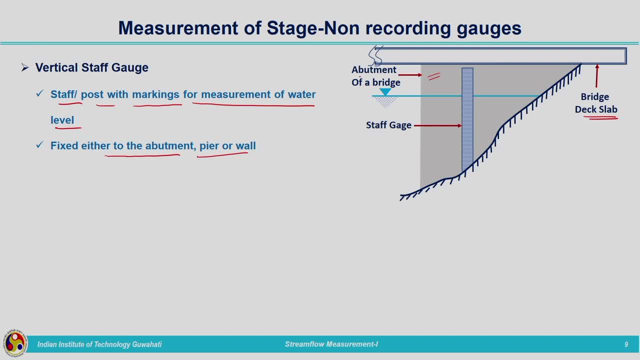 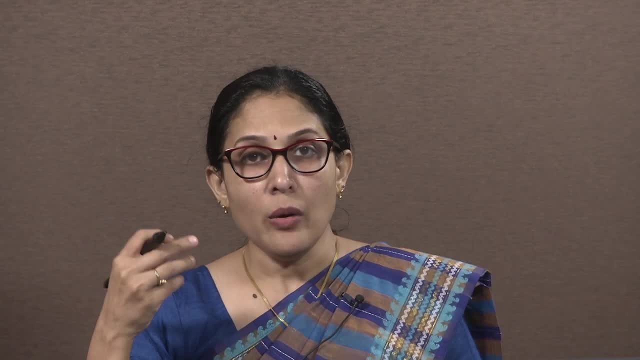 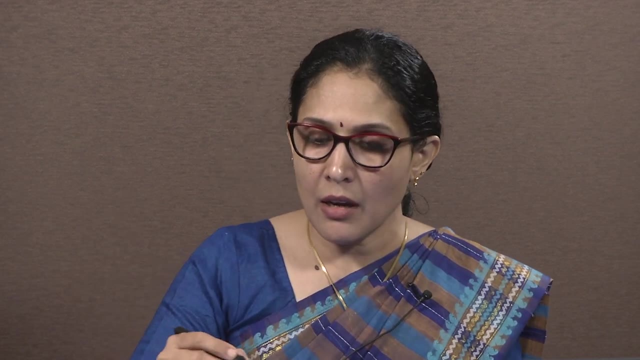 this is our staff gauge that is fixed to the abutment of the bridge, sometimes to the abutment of the bridge or sometimes to the bridge pier or any other hydraulic structure. it will be fixed. half gauge will be fixed on to that and we can measure the water surface elevation here. in this case this is the water surface. 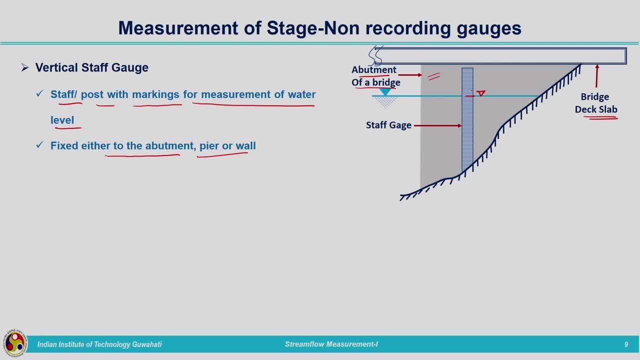 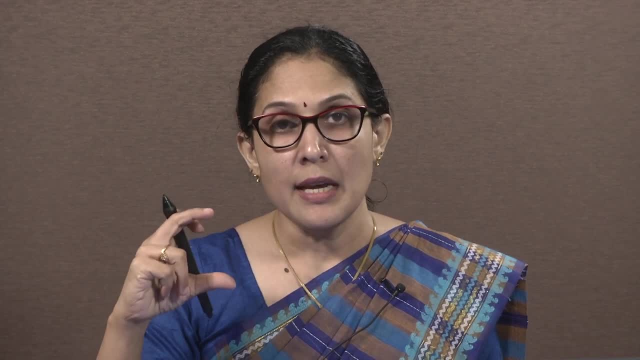 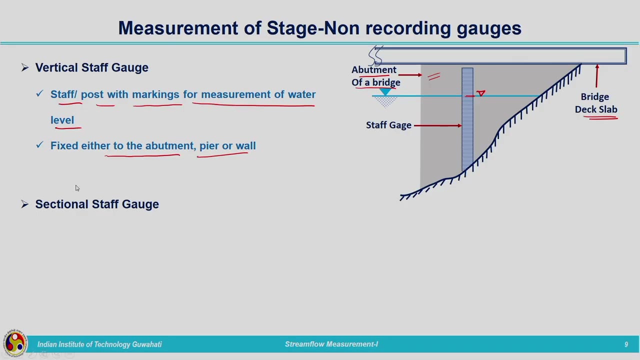 elevation that can be read from the staff gauge. so how much is the depth of water level or how much is the stage value of stage that can be observed from this staff gauge. Second one is the sectional staff gauge. This is also staff gauge. Sometimes it may not. 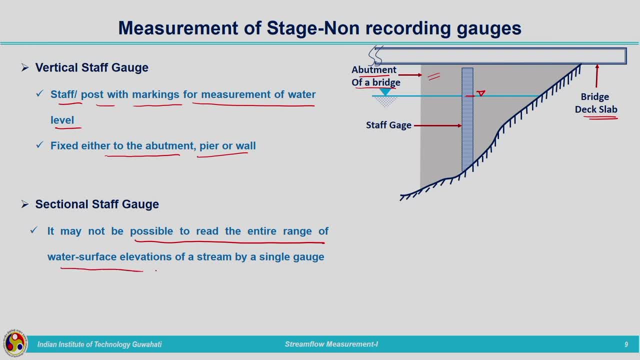 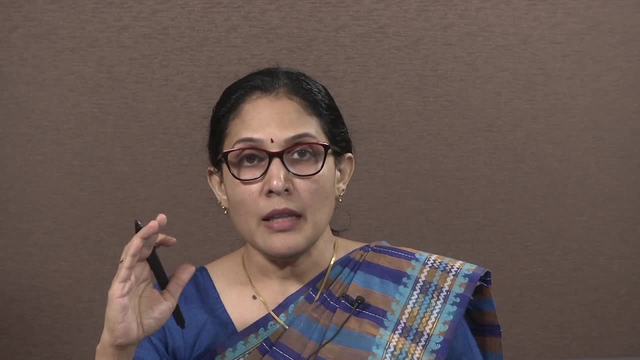 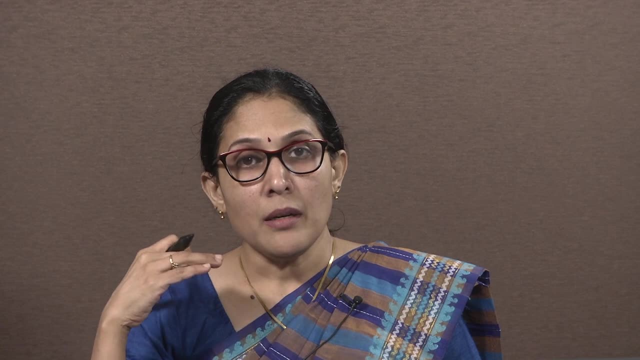 be possible to read the entire range of water surface elevations of a stream by single gauge. You can imagine a large river in that during the lean period, that is, summer season, water level will be very low, But on contrary to that, during the monsoon season water level will be very high. 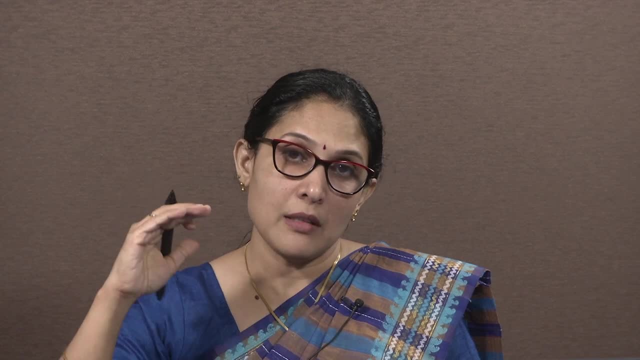 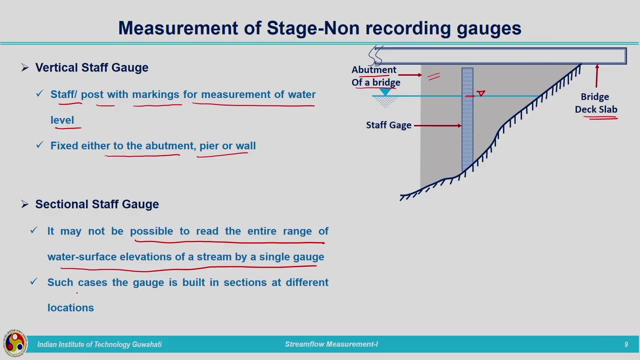 So measuring these much of water level, that is, high water level and low water level, by means of single staff may not be possible always. In such cases. the gauge is built in sections at different locations. It can be visualized by means of a schematic diagram. 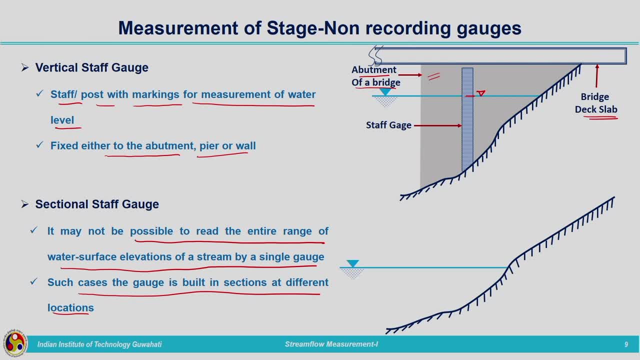 This is the riverbed and we are having the water level at particular season up to this, and different staff gauges are placed in the river like this. So during the high flood time, we may be having water level up to this level, So at that time this particular staff will be giving us the 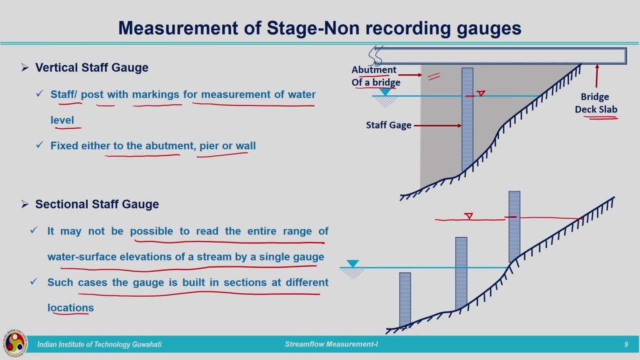 readings corresponding to water level, And some other season water level will be up to this level And we can make use of this gauge, which is present. in between And during lean period, water level will be very low. in reverse, the water level will be very low. 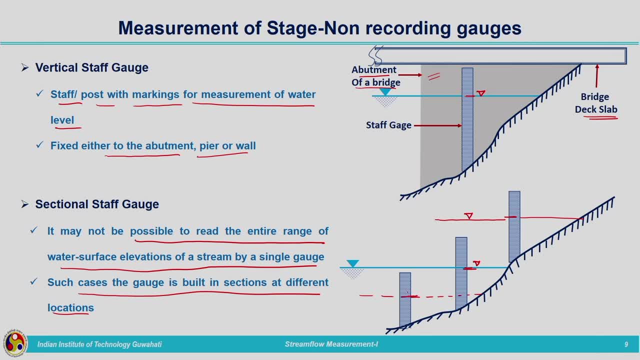 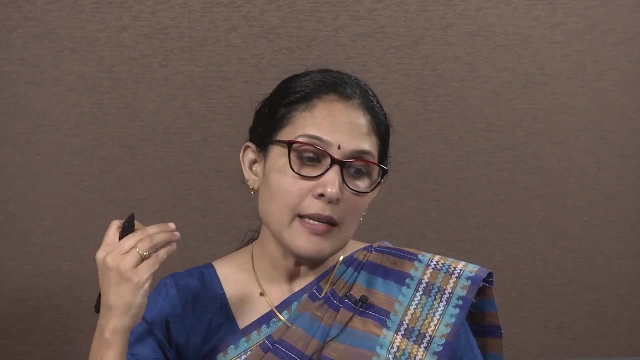 And we can make use of the one which is corresponding to that particular level. So that way, sometimes single staff won't be serving the purpose. So we will be providing intermittent staffs in order to measure the water level in all the seasons And, in addition to these type of vertical staff gauge, sometimes we will 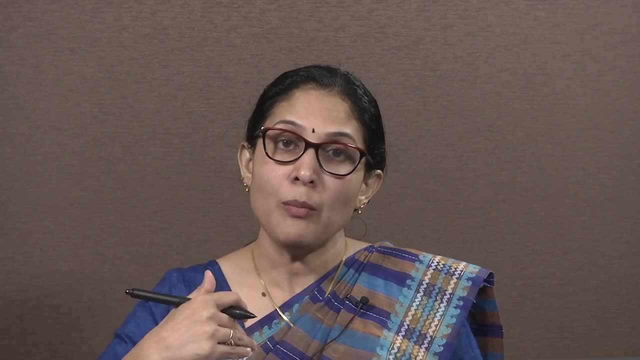 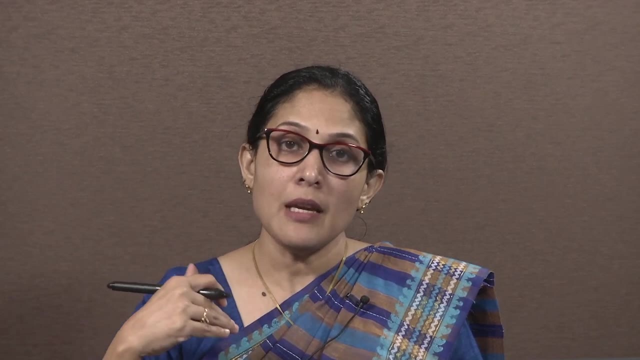 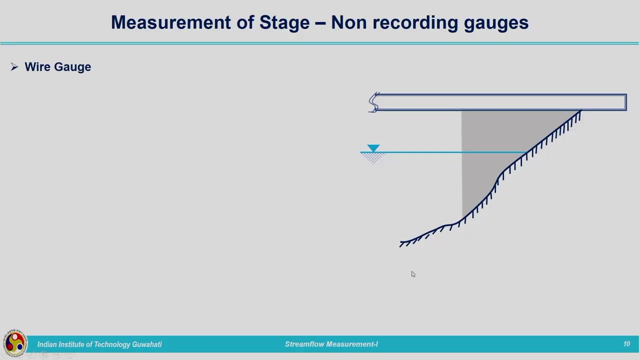 be placing in an inclined way, also with a bed it will be attached, and by making use of the, by knowing the angle of inclination which the staff is making, we can find out the depth of water within the stream. Next one is the wire gauge. this is again the 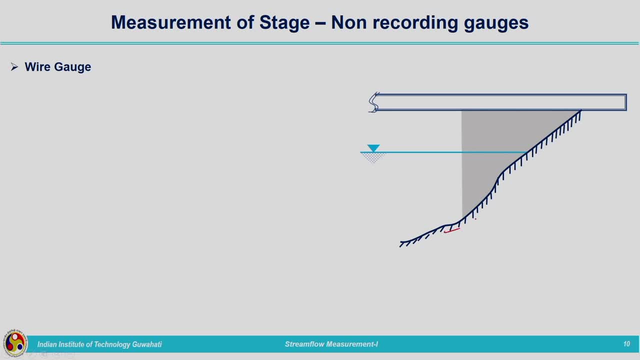 same figure. we are having the river bed stream is present, water level is up to this level and we are having the bridge abatement and in this is the bridge deck slab. In this what how the measurement is done. we are having a gauge drum of the gauge present. 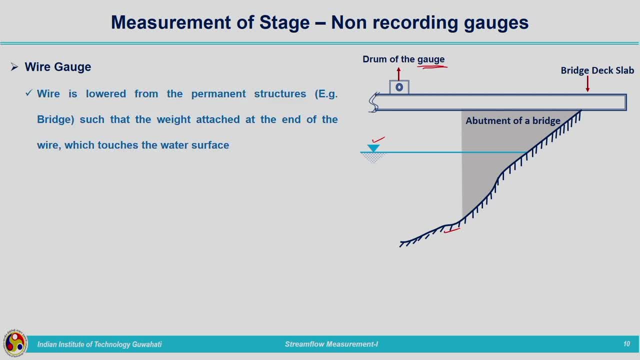 over the deck slab and from there the wire is lowered from the permanent structure, such as bridge, such that the weight attached at the end of the wire will be touching the water surface, That is, the wire is lowered from the bridge like this, and here at the bottom will be having 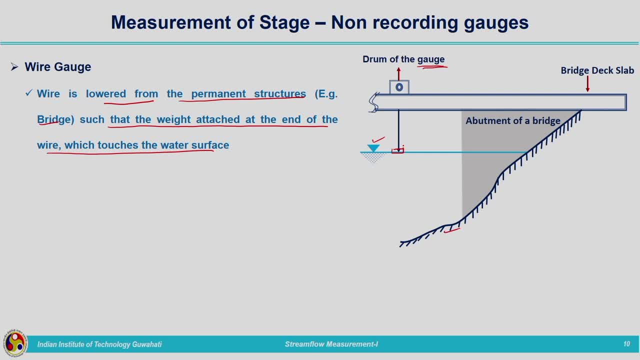 a weight attached to it. that weight will be touching on the water surface. This wire gauge is lowered from the permanent structure such as bridge, And the length of the wire coming out of the drum of the gauge is read by a mechanical counter attached to the reel on. 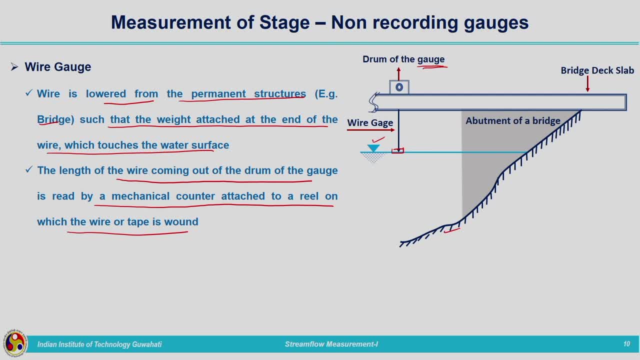 which the wire or tape is wound And the length of the wire coming out of the drum of the gauge is read by a mechanical counter attached to the reel on which the wire or tape is wound. There is a reel on which the wire is wound and this winding of the reel is done from. 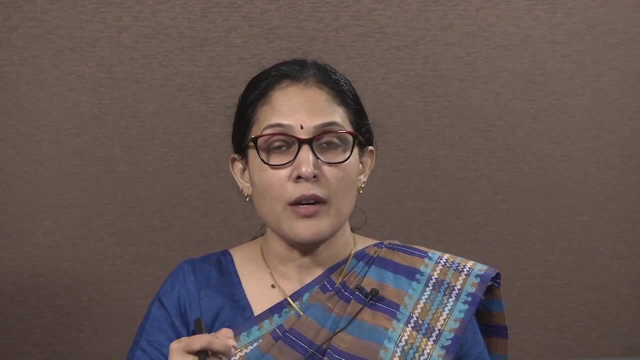 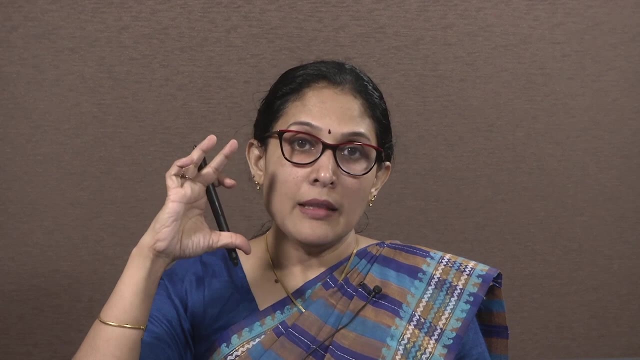 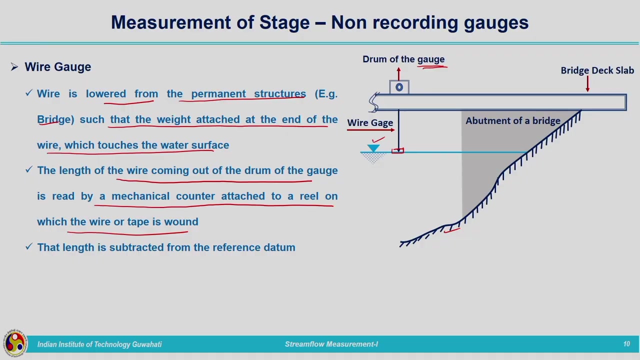 there. how much is the length of the wire which is lowered so that the weight is touching the water surface? that much length will be measured and that will be giving us the depth of the water level from the arbitrary datum And if we subtract that length from the reference. 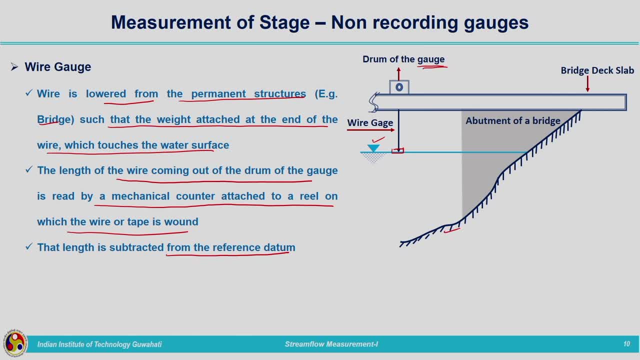 datum we will get the water depth. So, from this particular point to water level, how much is the depth we will be getting? and from the reference datum, from this datum level, how much is the level from that? we will be subtracting this d so that we will get the water level at this particular point, And 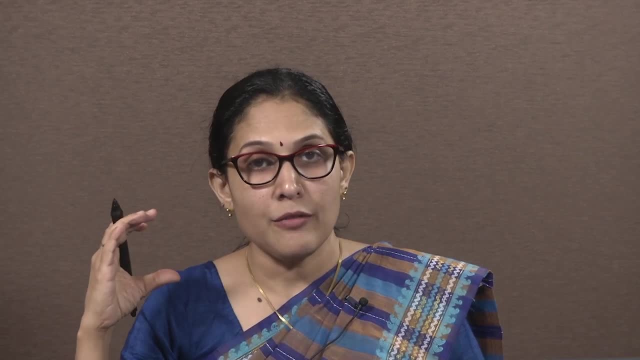 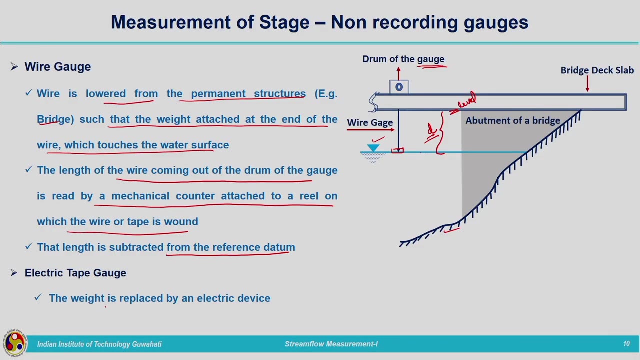 depending upon the position of the weight, we can get different water levels. Next one is the electric tape gauge. In this case the weight is replaced by an electric device. here this particular weight is replaced by an electric device. rest of the mechanism is same as that of the wire. 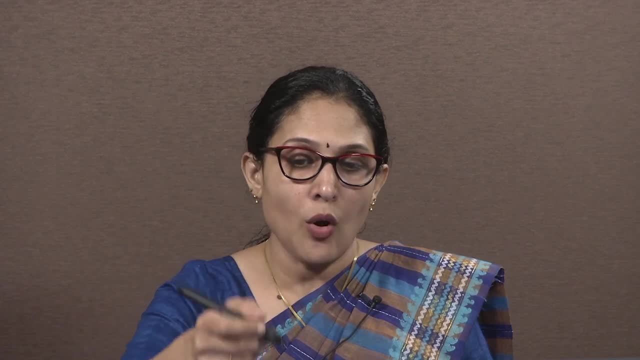 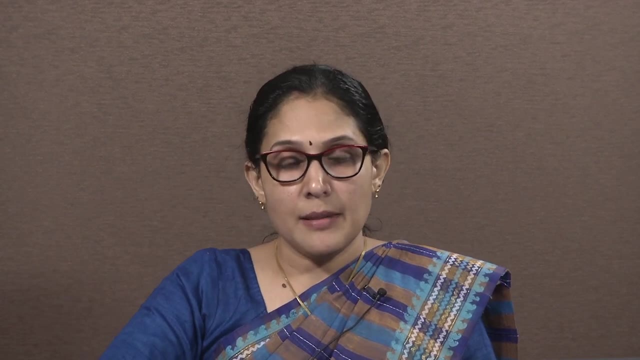 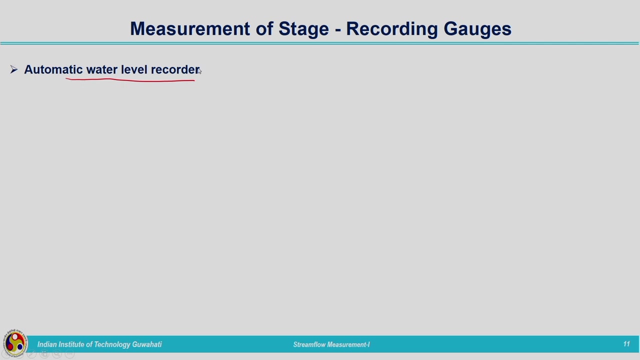 gauge wire is lowered from the top, from the drum of the gauge, and this weight is replaced by means of a, an electric device. Now, next one is the recording gauge: automatic water level recorder. So in this case manually, we do not have to measure automatically it. 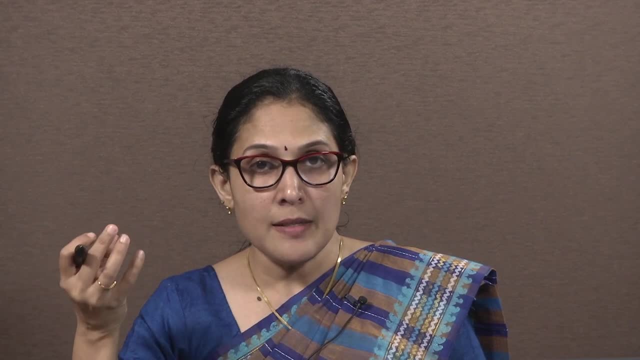 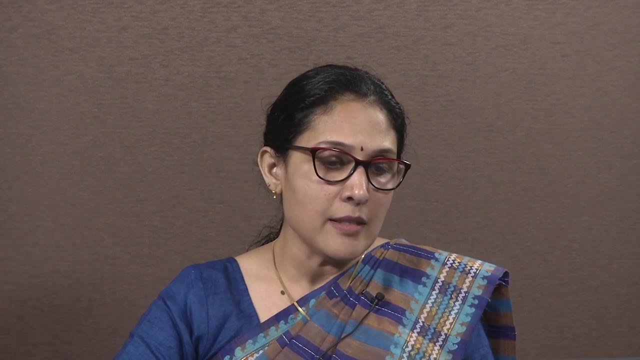 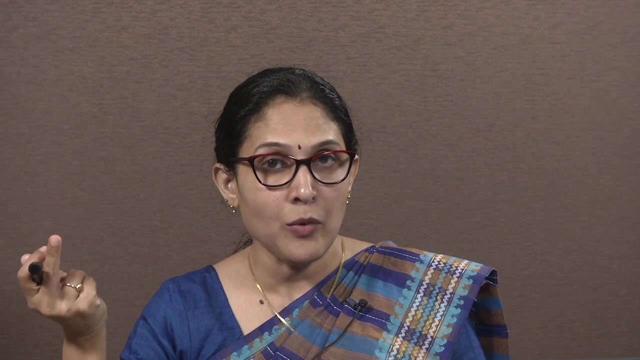 will be measuring the water depth, that is, there will be some data logger and that will be providing the data in the computer. So how the mechanism is, let us see that it measures water level continuously. In the case of manual measurement, whenever required, we will be doing it manually. but in this case, since it is automatic, it is recording. 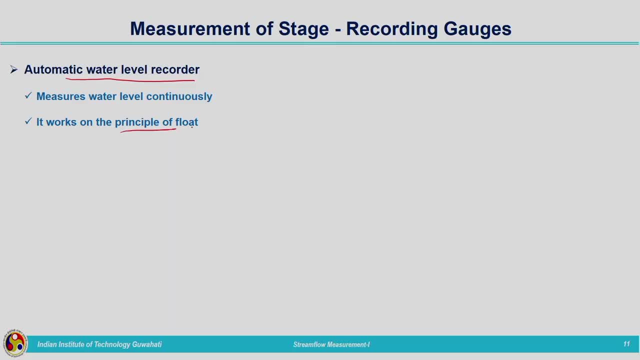 the water level continuously. It works on the principle of float and, again, schematically, we are having the stream, we are having the approach bridge, like this, And here, in this case, since it is a continuous measurement technique, continuous measurement of water level is taking place. we are having 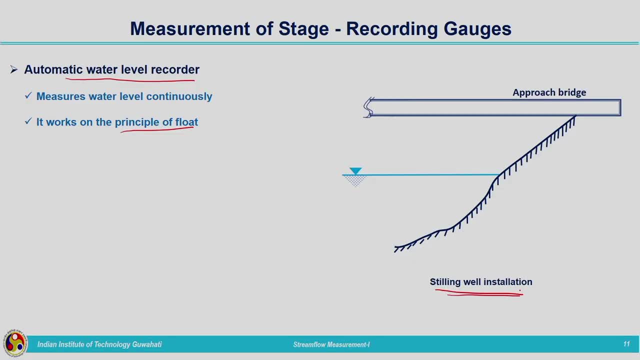 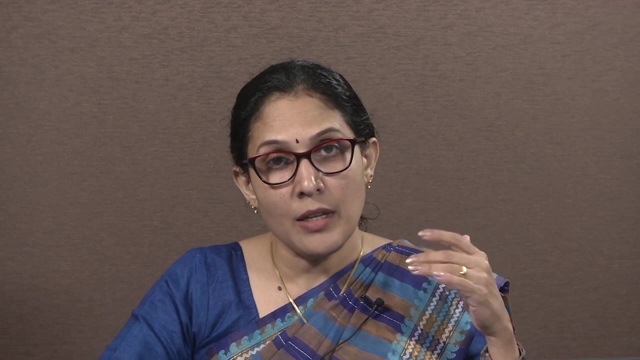 a stilling well installation to protect the instruments. So this is the stilling well installation and we are having an intake. well Within that we will be having one gauge for the manual measurement and also one automatic water level measurement mechanism. So this is our stage gauge, that is, water level measurement. 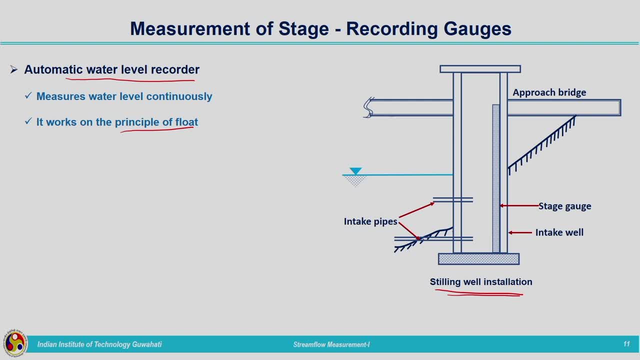 manually can be done and we will be having intake pipes. Two intake pipes are provided so that water will be entering into the intake well through those intake pipes and the water level which is present on the stream will be maintained within the intake well also, 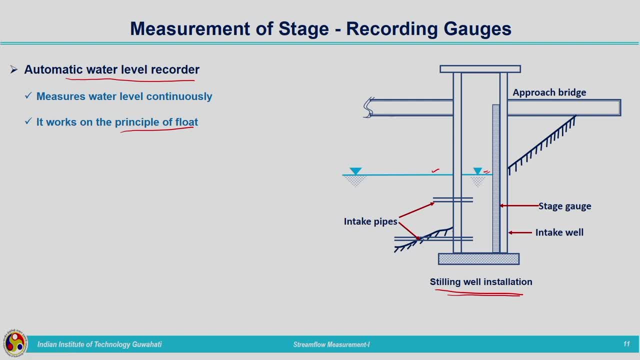 Now how this water level measurement is done automatically. We are having a recorder like this: Pulley weight arrangement is there And a surface float is connected to one end of the wire passing through this recorder. You can see this is a wire through this pulley. it is moving At one end of the wire there. 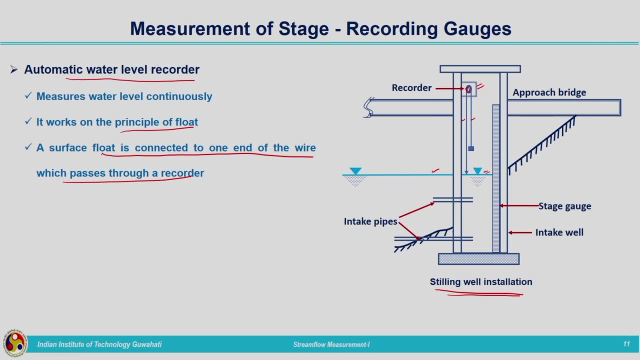 is a float which is present and, depending on the water level, this float will be moving up or getting lowered. if the water level is increasing, the float will be moving up. based on that, this weight will be moving down. so this movement of this float and the weight will be noted down by the recorder. 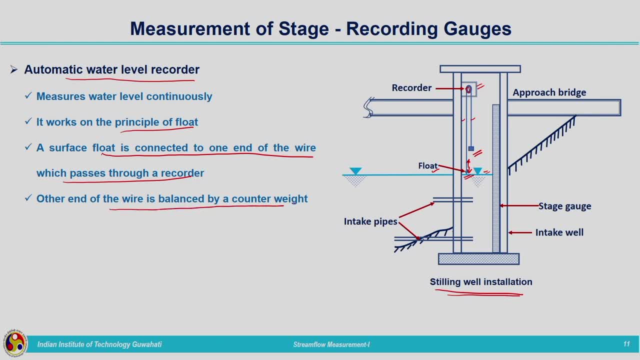 so this float one end of the wire is balanced by the counter weight that is marked over there, and the fluctuations in water surface level make the float and drop, along with the wheel of the recorder, to move, so, as the pulley rotates, the stylus or the pen, which is present over there, 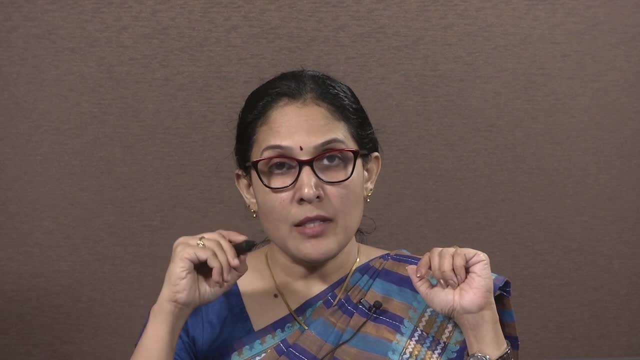 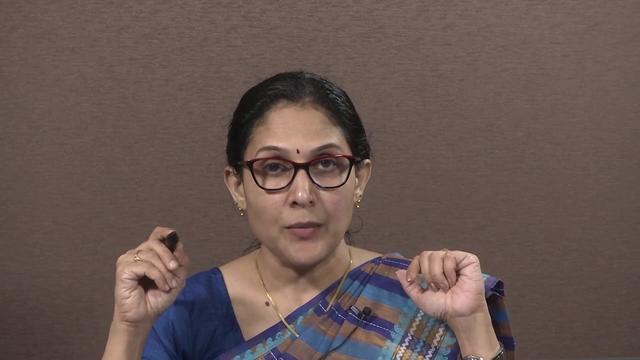 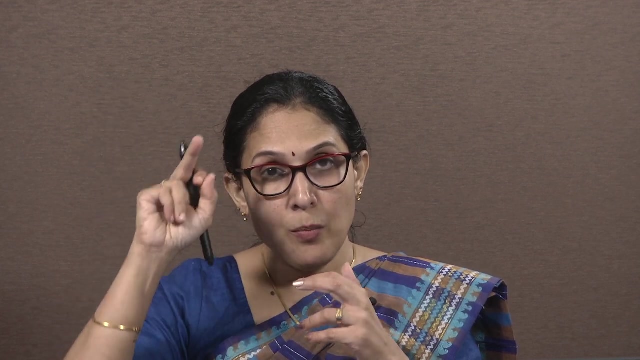 will be recording the movement so based on that we can understand how much is the variation taking place in the water surface or water level. so whenever the water level is rising, float will be rising and the weight will be lowering, so pulley action will be taking place. 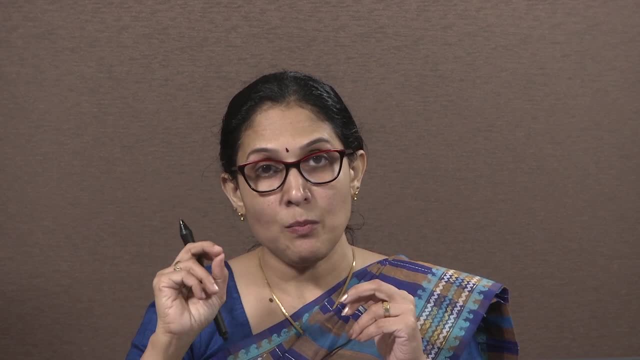 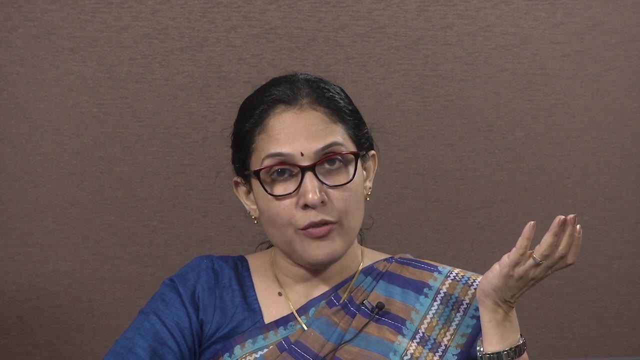 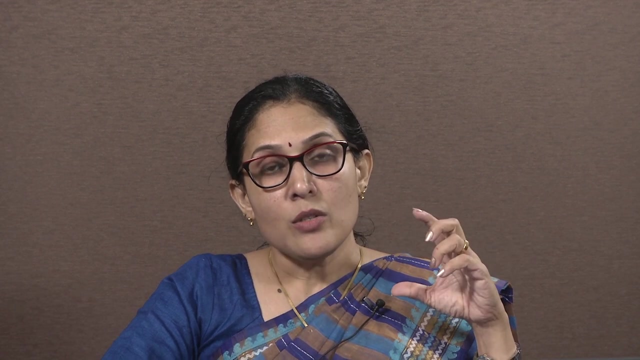 there and the stylus or the pen which is attached to this pulley will be noting down the water level readings. so that much about the measurement of stage, and different techniques are there other than this ultrasound depth measurement meter. so those type of measuring techniques, the sound waves, will be sent to the bottom of the 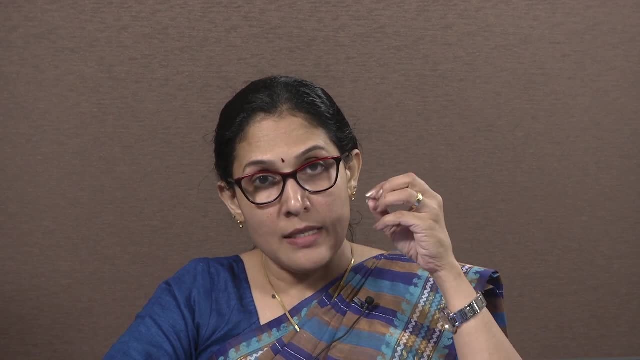 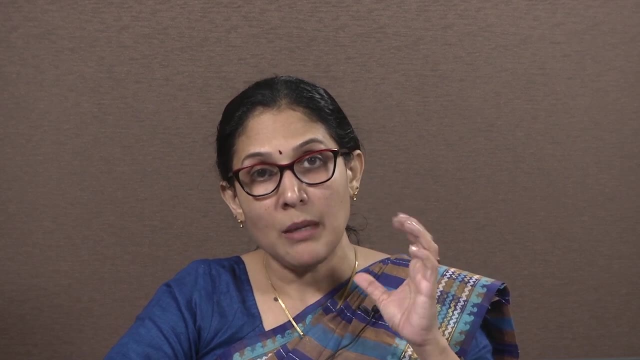 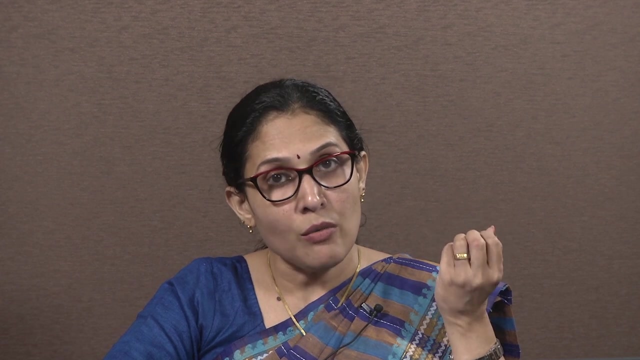 river and one transducer will be sending the signal and the same will be collecting that. the time taken for this waves to travel to the bottom- and coming back to the transducer, will be noted down and based on that we can get how much is the depth of water and also velocity of water. 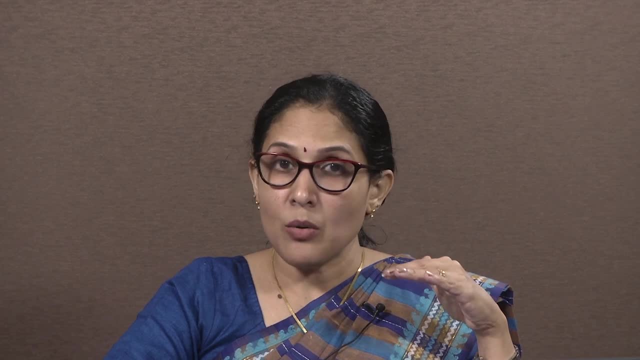 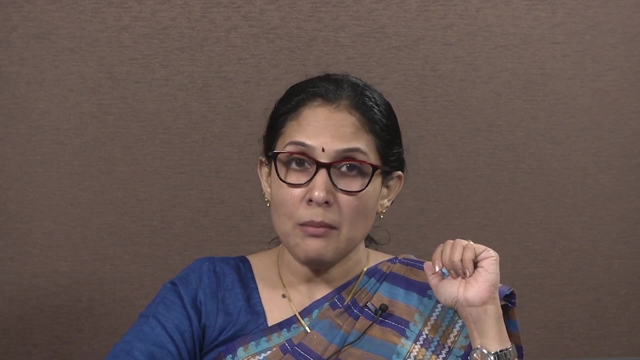 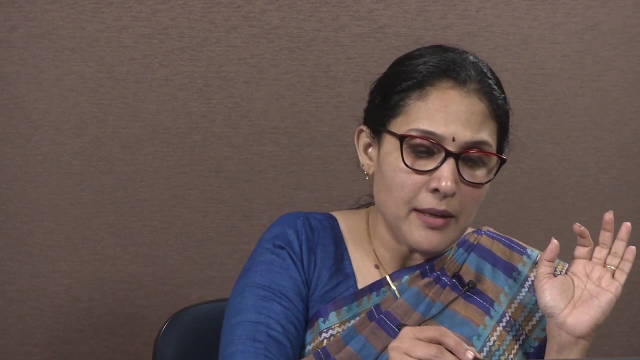 all these things can be understood here. i have explained only the conventional ways of measuring stage or the water level. now let us move on to the velocity measurement techniques. very commonly used velocity measuring technique is by means of current meter. it measures the velocity at a point in the flow cross section, so current meter is the one. 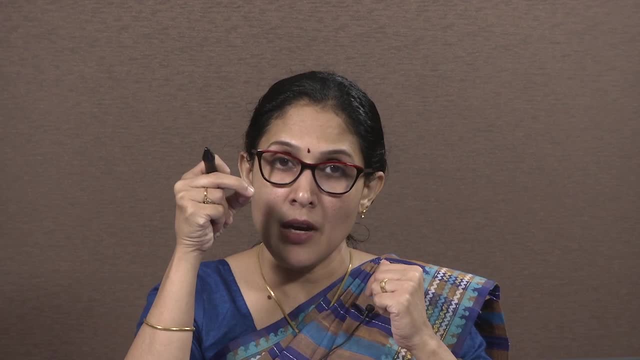 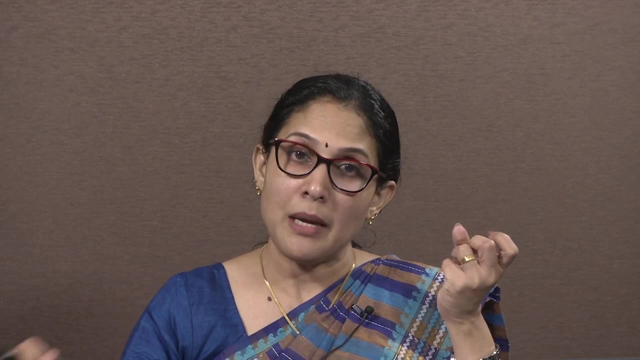 which is measuring the velocity at a particular point where we are positioning this current meter based on that velocity at that particular point, will be obtained by making use of current meter. so when i was discussing about average velocity, i told you, in the case where i was doing analysis of the current meter better at that mode value, which 레黙ים. 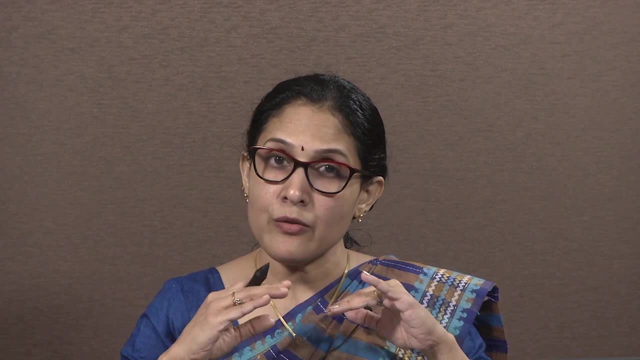 is equal to ю, the value mat, not the expression of the velocity that may be achieved. so maximum velocity on the water surface velocity: 170 Mach n, plus where we measure theid velocity case of shallow rivers, we need to measure the velocity at a depth of 0.6 times the depth 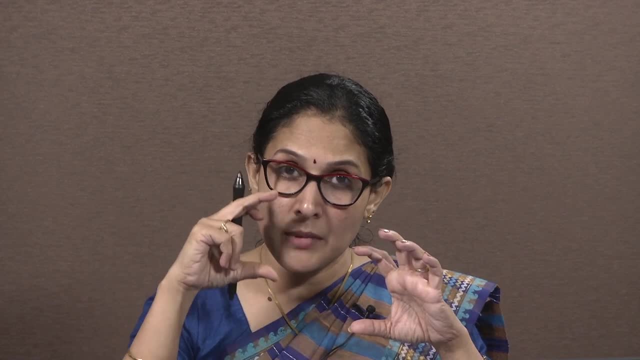 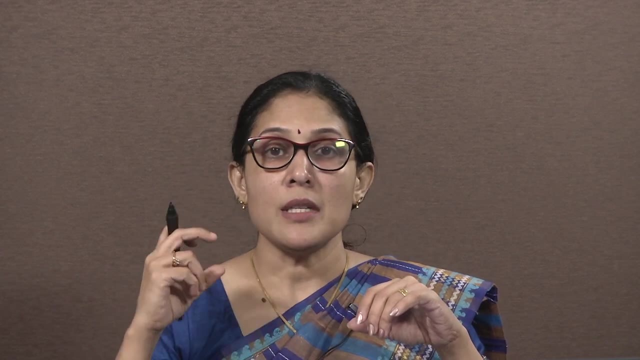 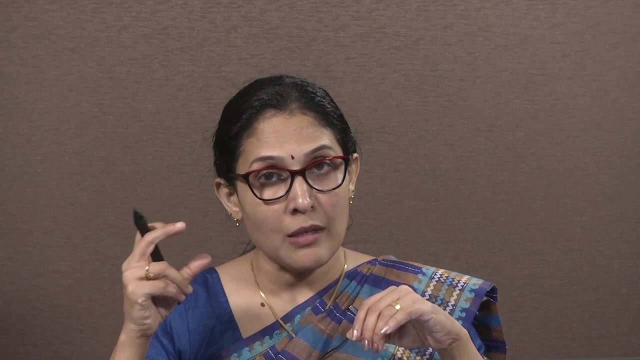 of flow. So, at the locations, if the depth is y 0.65, we will be positioning the current meter So that we can get the velocity at that particular depth. In the similar way, whichever be the depth we are in need of that, whichever be the depth at which the velocity, 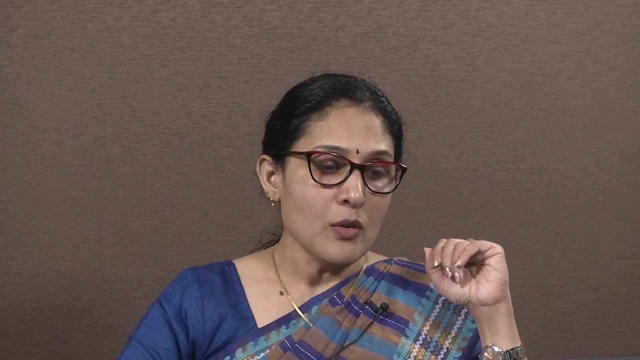 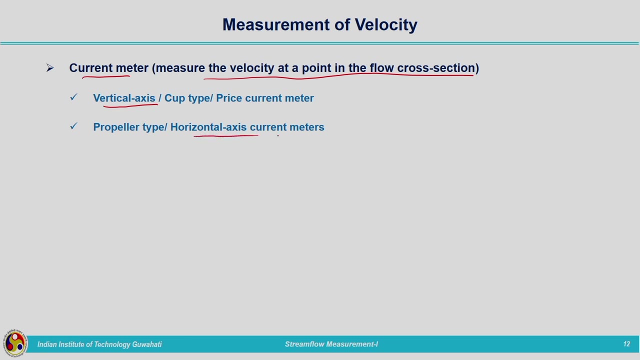 is required, we will be positioning the current meter. So different types of current meters are the vertical axis current meter and also horizontal axis current meter. Vertical axis current meter is also known as cup type current meter, commonly termed as price current meter, And the horizontal axis current meter is the propeller type current meter. So these are: 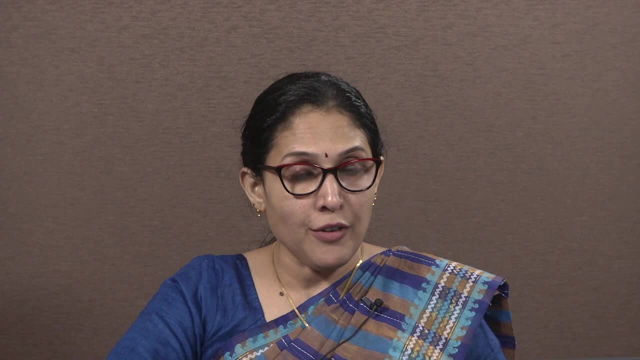 the two types of current meters which are commonly used in the field. Now, other way to measure the velocity: at a depth of 0.6 times the depth of flow, we are measuring the current meter service. The other way of measuring velocity is by means. 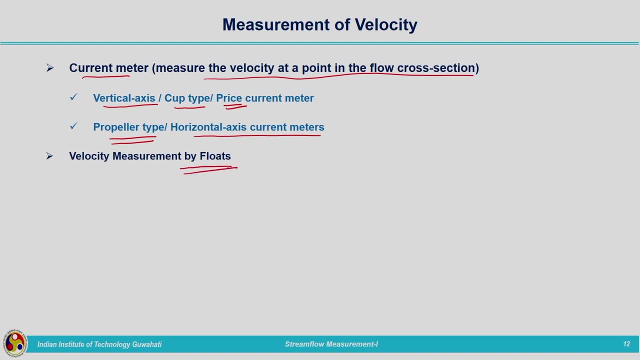 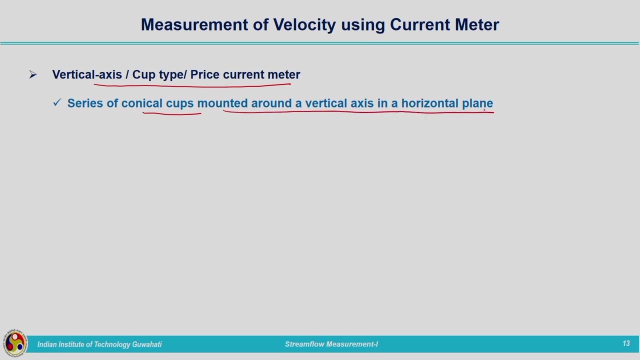 of floats. we can make use of floats for the measurement of velocity also. So two ways are the: by means of current meter and also by means of floats. Let us look into the case of current meter first is the vertical axis cup type, price, current meter Series of conical cup bounded around a vertical axis in a horizontal plane. So this is the vertical axis current meter. This is a series of conical cups, This is a series of plus and minus and minus conical types. So the vertical axis current meter is the period of the down payment on this JuliusGAN, which makes Кон separated SAL Easter. 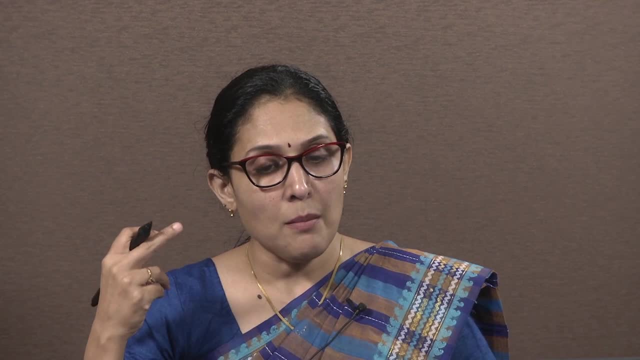 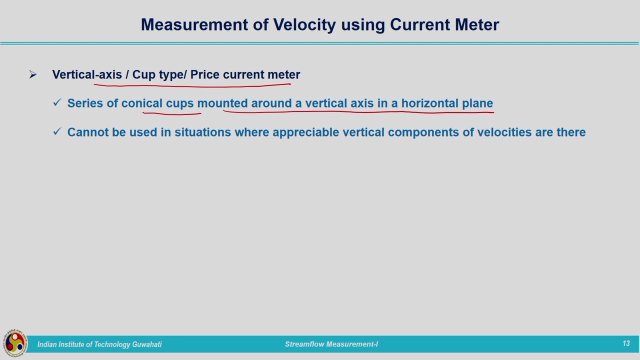 is current meter. So in this series of cups are mounted around a vertical axis in a horizontal plane, And the disadvantage in this case is that it cannot be used in situations where appreciable vertical components of velocities are there, If vertical components of velocities are. 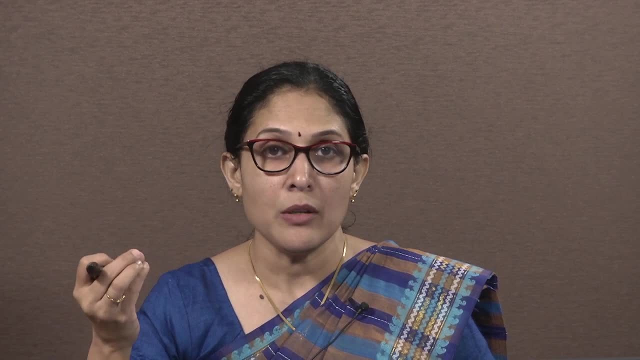 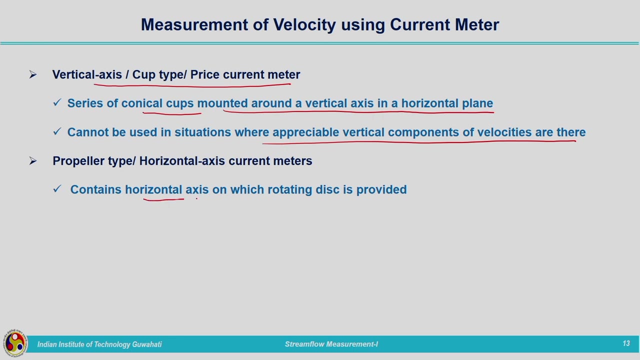 there, it will not be giving us the accurate measurement of velocity. Second, one is the propeller type or horizontal axis current meter. It contains horizontal axis on which the rotating disc is provided. Only difference is that in this case it is the horizontal axis. On the other hand, 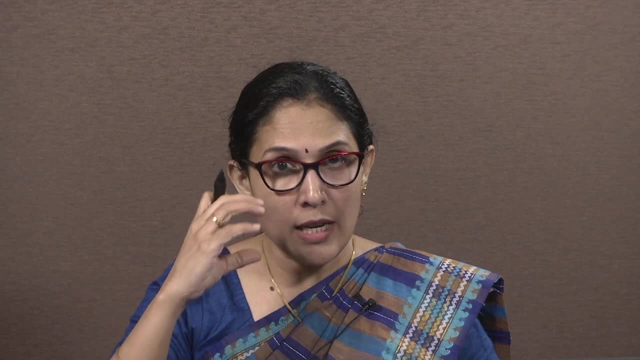 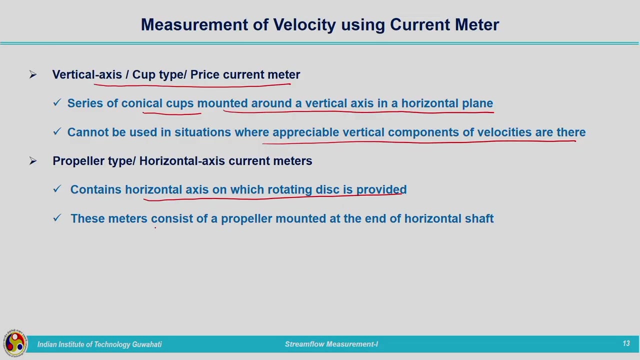 in the case of vertical axis current meter, the conical cups are mounted on a vertical axis in a horizontal plane, And in the case of propeller type, these meters consist of a propeller mounted at the end of horizontal shaft, And these are robust and not affected by. 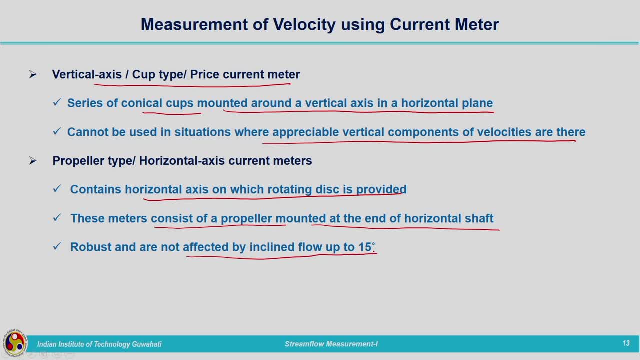 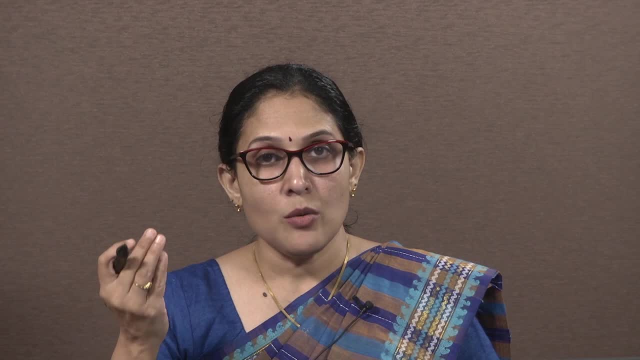 the current. So in this case the propeller type or horizontal axis current meter contains horizontal inclined flow up to 15 degree. These are horizontal axis current meters. Even for some inclination it will give accurate measurements. So two different types of current meters. One is 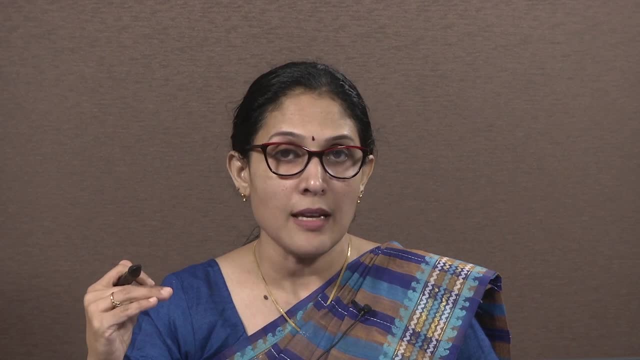 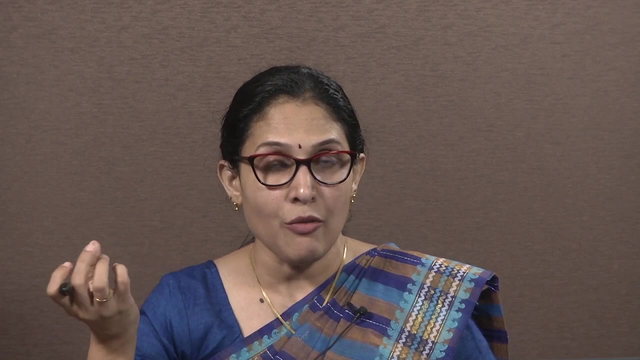 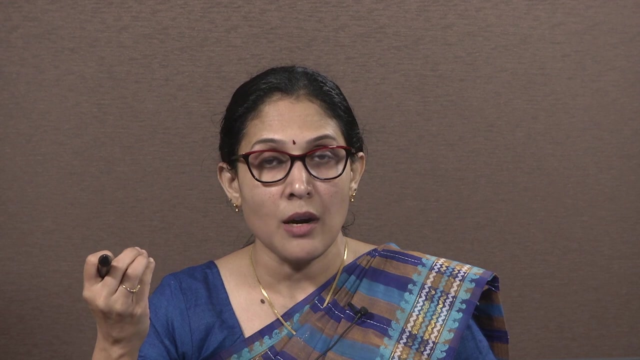 the vertical axis current meter and the other one is the horizontal axis current meter, So conical cups are attached to it. The movement of the cups due to the velocity of flow will be noted down. That rotations per minute or rotations per second will be noted down And those rotations will be converted into the velocity. So for that the 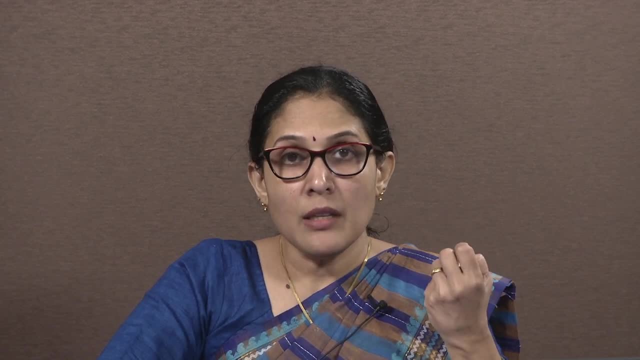 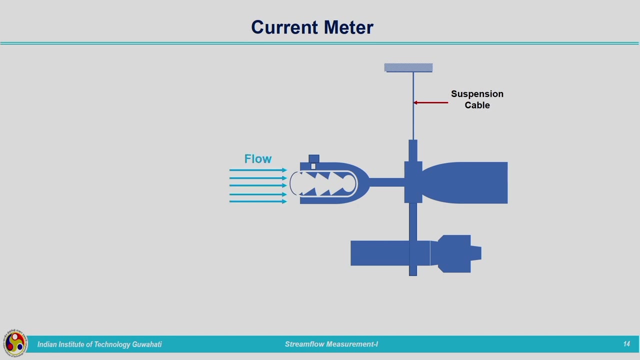 current meter will be having certain formula to calculate the velocity. This is the schematic representation of a current meter. We are having suspension cable From there. the current meter is suspended, A flow is taking place in this direction And because of this flow, what will happen? the cups. 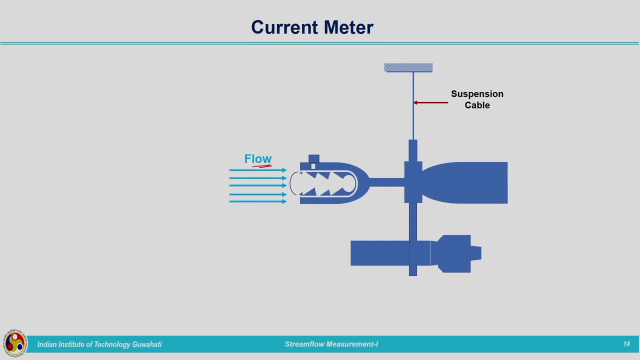 which are attached to the current meter, will be converted into the velocity. So, for that, the current meter will be rotating. So the cups are present over here, Different number of cups are there, And these cups, due to the movement of flow, due to the velocity of flow, these cups will be rotating And 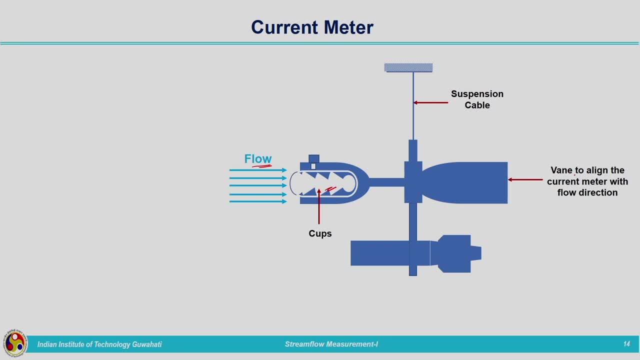 on the other side- other side of the current meter- there is a vane present to align the current meter with the flow direction. This is the vane which is there in the current meter. The main purpose of this vane is to make the current meter or to align the current meter in accordance with the flow. 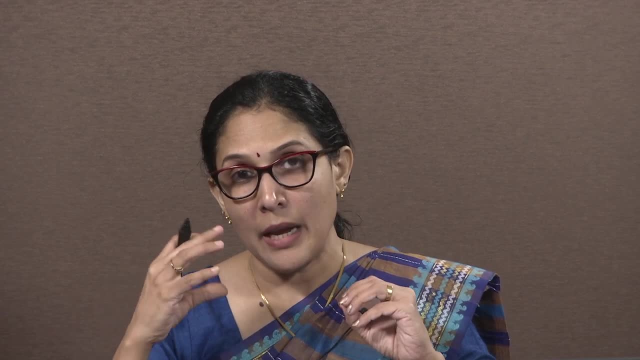 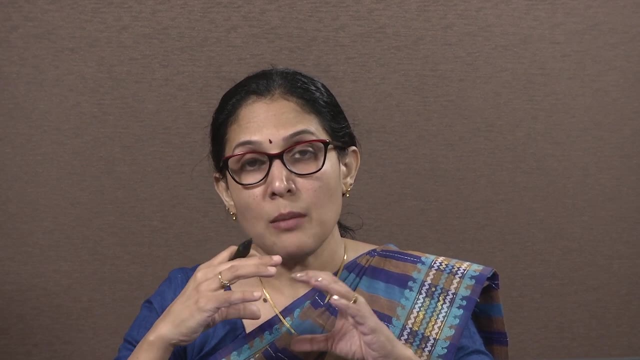 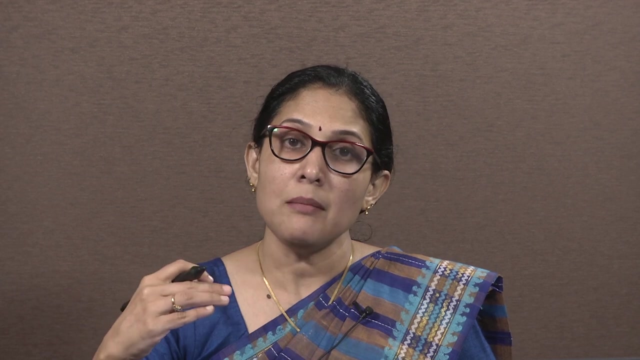 That is why this vane is always made of some streamlined body, Some shape similar to that of a fish. So those type of streamlined structure will be provided for this vane And this will be aligning the current meter in proper position with the stream flow, And here we are having a balancing. 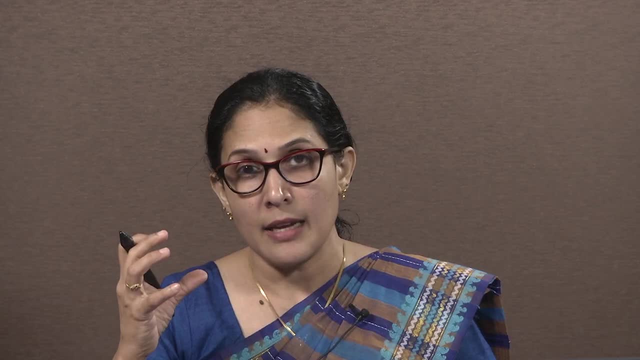 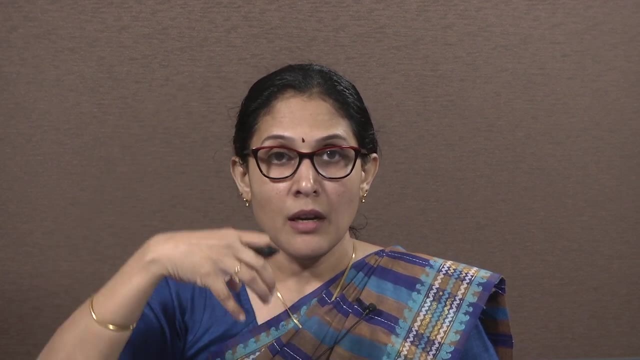 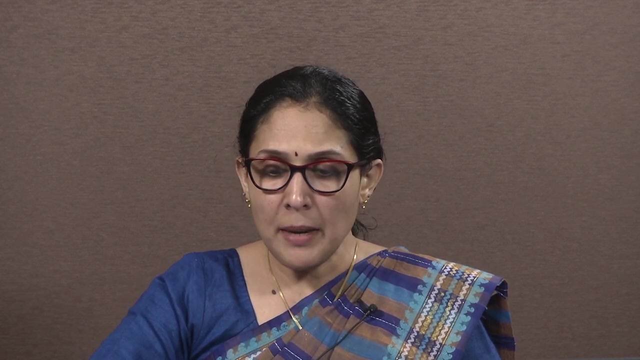 weight provided. What is the role of this balancing weight? is that this will be providing when we are suspending the current meter. it has to be in position for that. we need to provide certain weight at the bottom. That is the balancing weight. So here we are having a counting mechanism. This 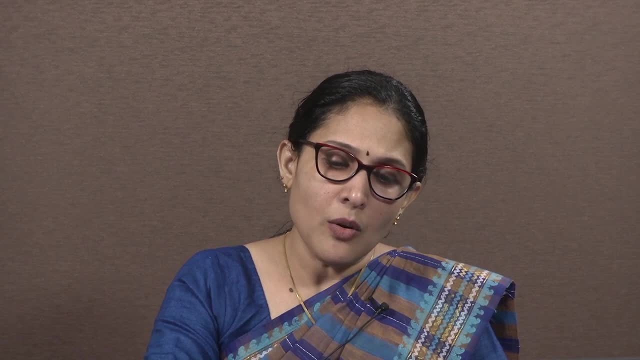 counting mechanism will be making the measurement, or the number of rotations which the cups are in, Which means that is the timing for the cup to move, And also there isimore of rotations for each of these various of the cups. So that will be Barb singular rotation. that is all, Then. 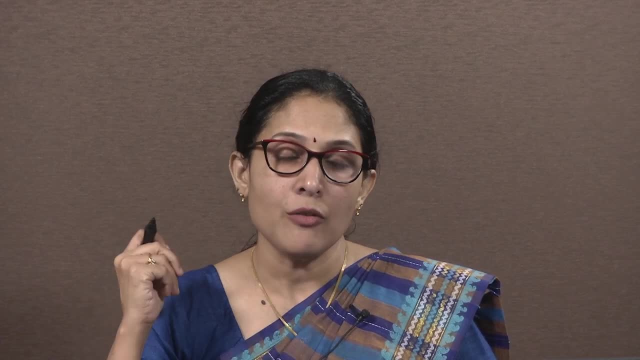 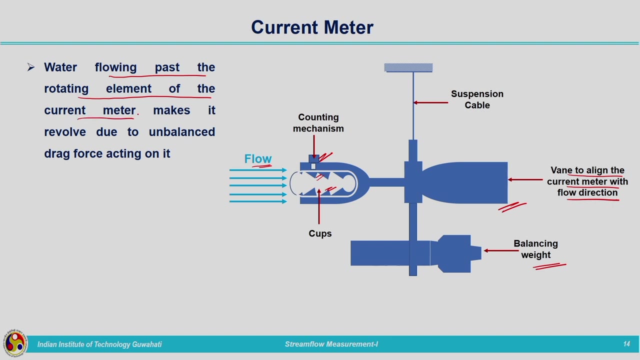 the measurement겨 from the rotor foot we weight, which is also being used for the cups. So part of flow that will be recorded by means of this counting mechanism. So water flowing past the rotating element of the current meter makes it revolve due to unbalanced drag force acting on it. 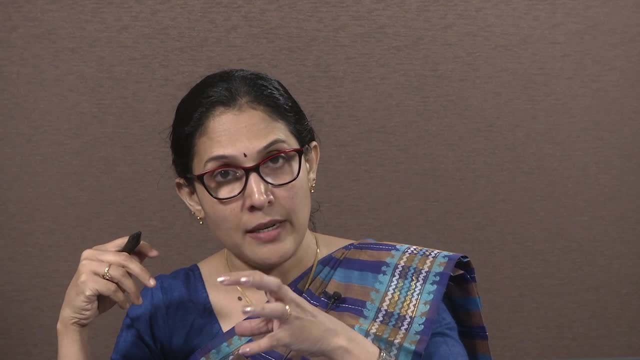 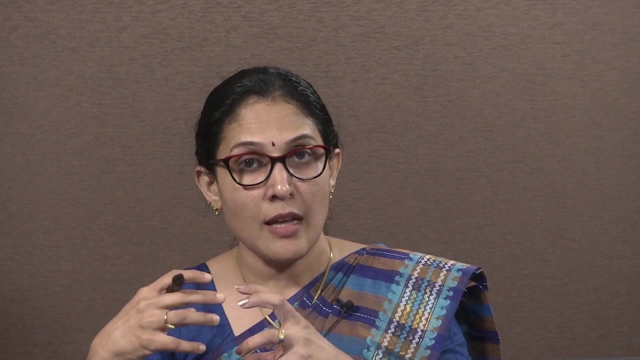 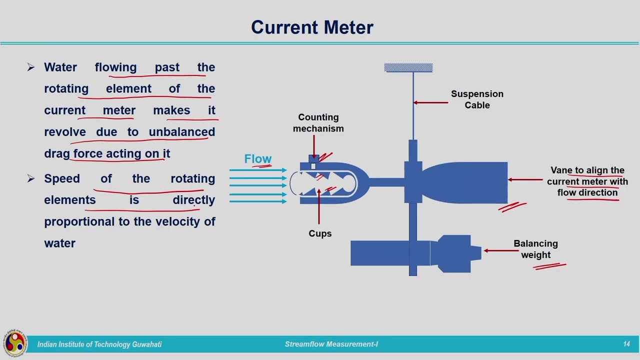 Water flow is there and based on that, there will be a drag force acting on that. because of that, this conical cups will be rotating. those rotations are of interest. that is recorded by means of the counting mechanism. So speed of these rotating elements is directly proportional to the velocity. 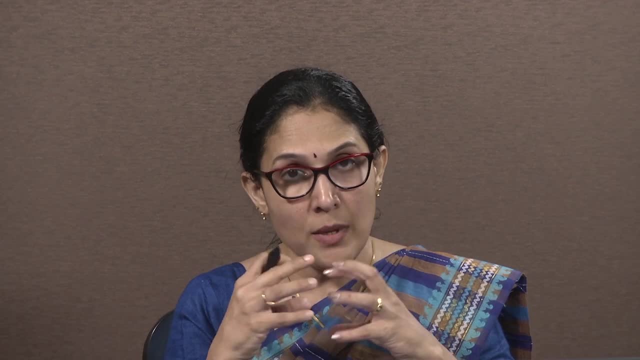 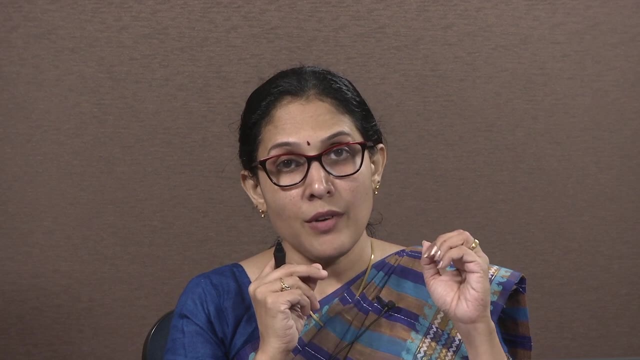 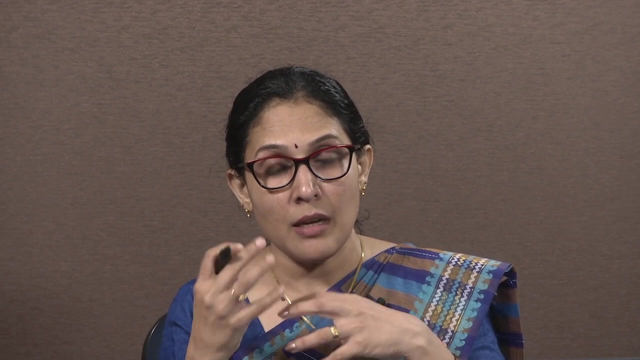 of water. that is the way in which it is related. How much is the speed with which the cups are rotating that determines the velocity of flow? If it is a very turbulent condition, then the rotation of the current meter cups or the conical cups will be at a higher rpm rotations per. 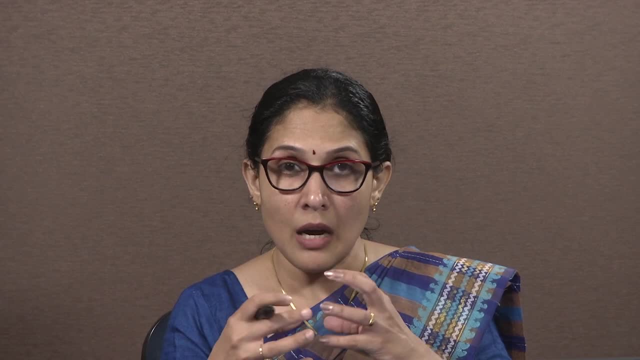 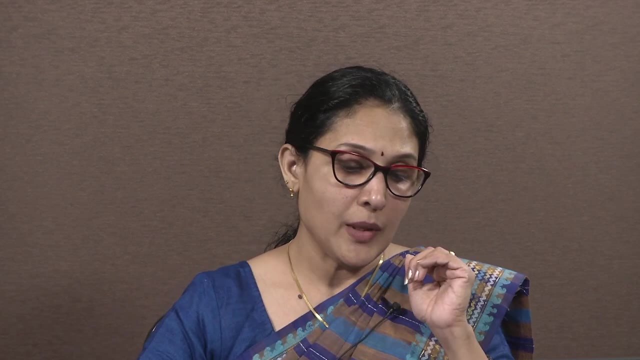 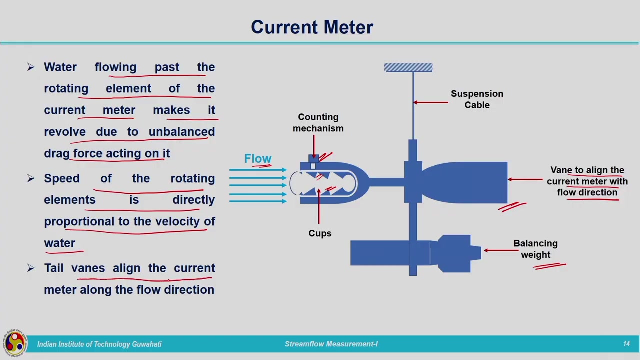 hour, Higher rotations per minute will be there. So, depending on the rpm or the, depending on the number of rotations, we will be getting the velocity of flow, because that velocity of flow is creating the rotations of these cups. These tail vanes align the current meter along. 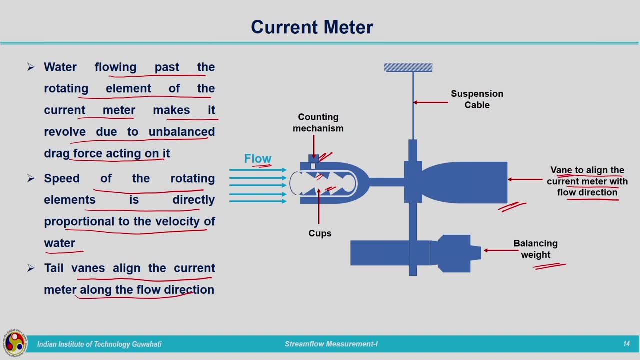 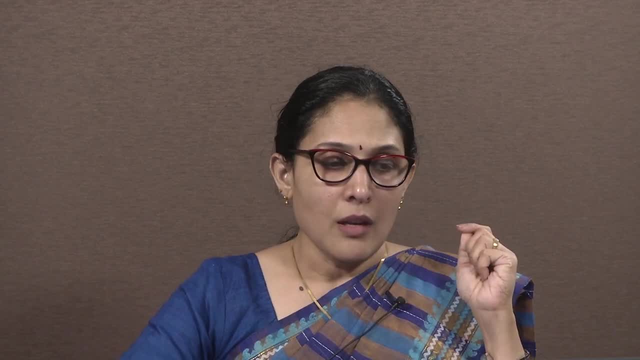 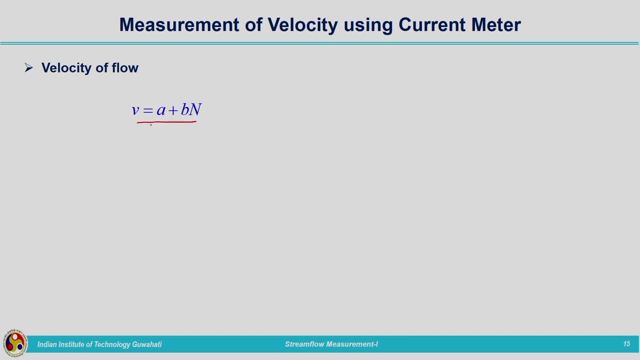 the flow direction. I have already told you these tail vanes will be having the shape of a streamlined body, so that the alignment will be proper along with the flow. Now, by using the current meter, how to measure the velocity of flow. Velocity of flow can be calculated by using: 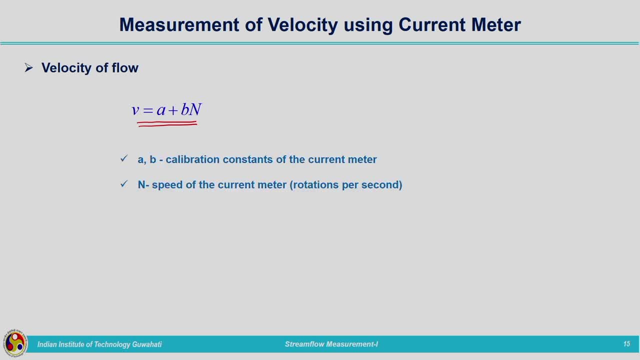 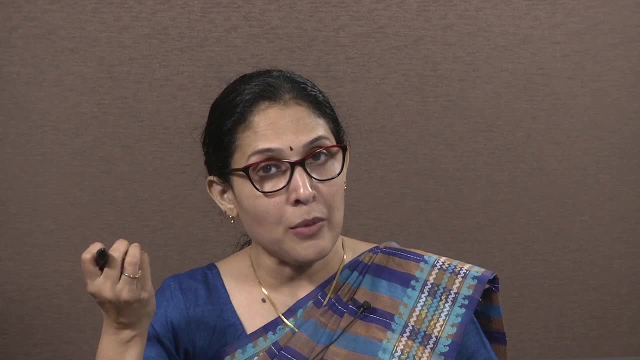 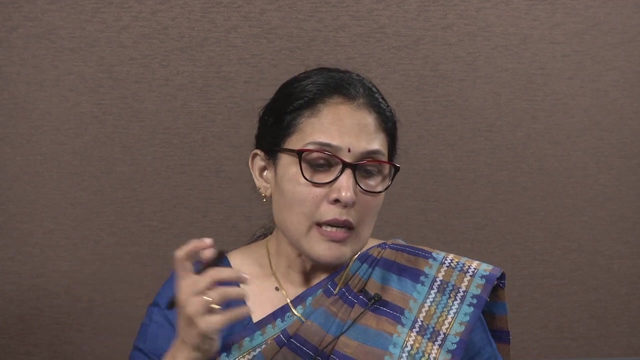 this formula V is equal to a plus b, n. In this a and b are the calibration constants of the current meter. This depends on the current meter. It will be provided in the manual itself. Sometimes we may have to go for calibration of the current meter. So capital N is giving us the speed of the current. 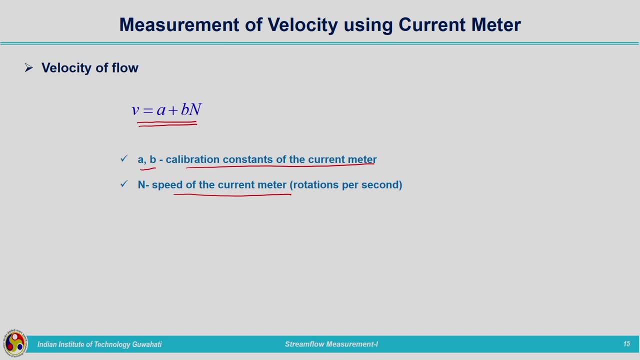 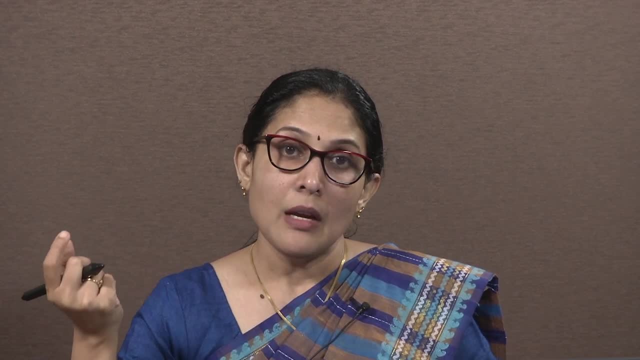 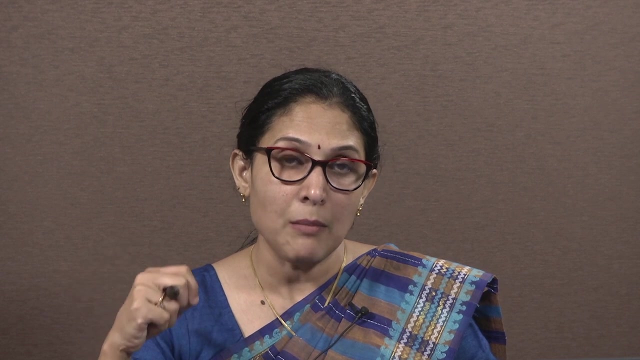 meter. that is rotations per second. If I take thisellenpointer and carefully take it, I will get a solution. this In this one second: how many rotations have been taken place for this conical cups? that will be noted by the counting mechanism if the rotations per second is available, RPM, rotations per minute or rotation per second is available. 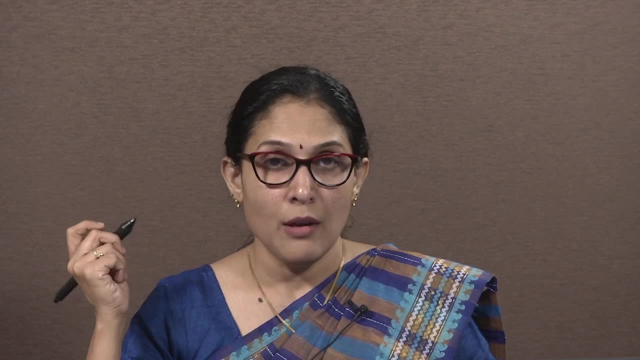 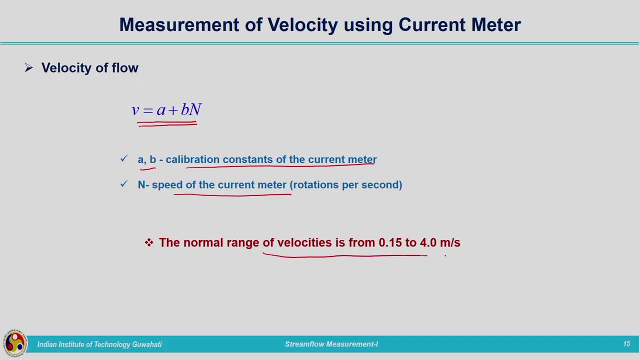 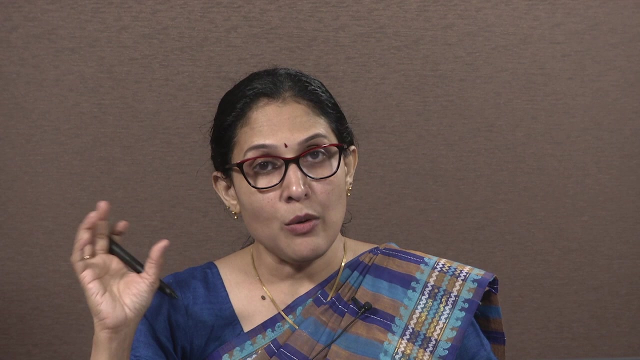 to us That can be utilized, along with the calibration constants, to get the velocity of the flow by making use of the current meter. the normal range of velocity is measured by current meter to 4 meters per second. Up to 4 meters per second. we can make stream velocity measurement by using 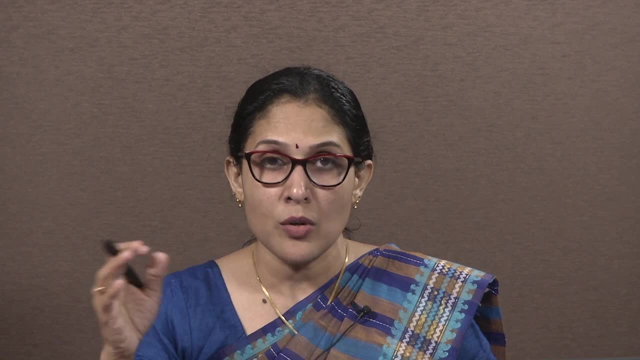 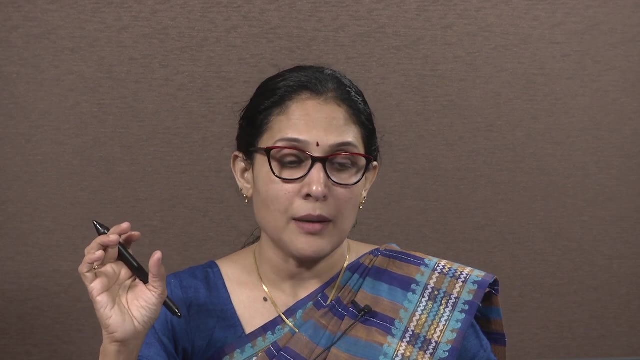 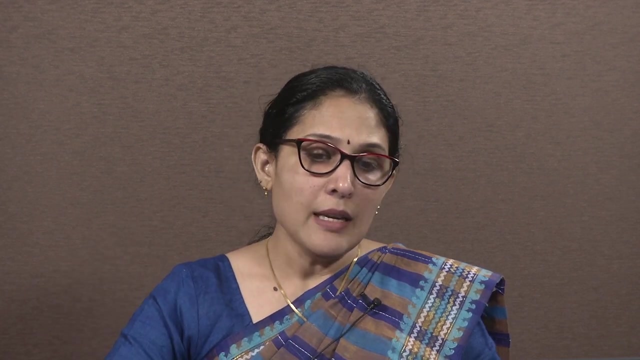 current meter, Any of this- vertical axis current meter or horizontal axis current meter. we can measure velocity up to within this range: 0.15 to 4 meter per second Formula, also similar to this: calibration constants will be different for different current meters. Next is the velocity. 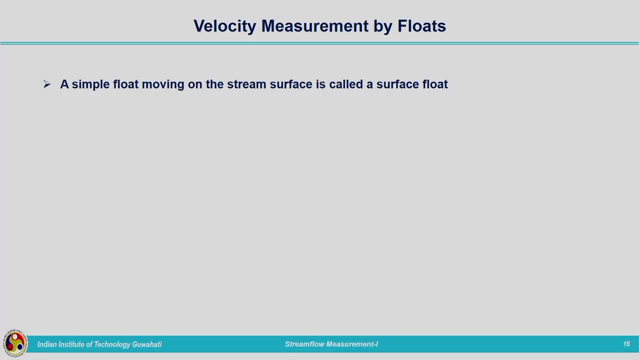 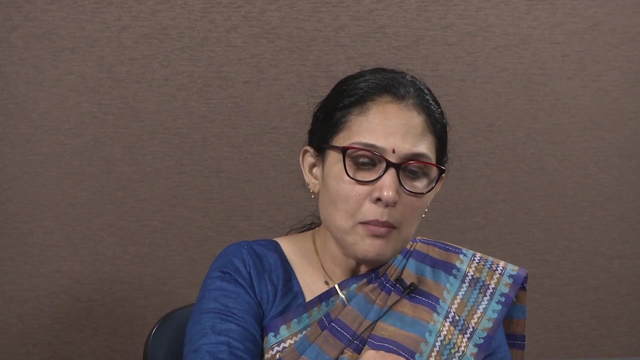 measurement by means of floats. So a simple float moving on the stream surface is called a surface float. Simple float which is moving, that is, a float is allowed to move on the surface of the water. that is called surface float. and time taken by the float to reach a known 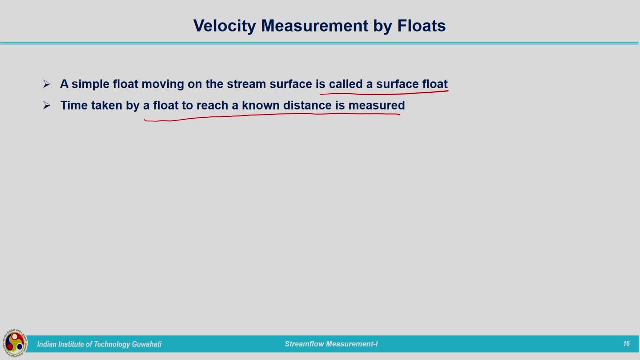 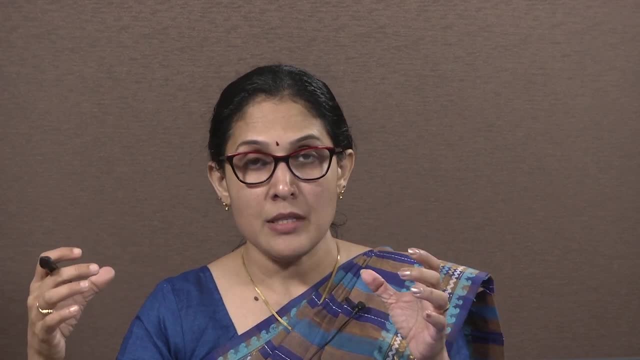 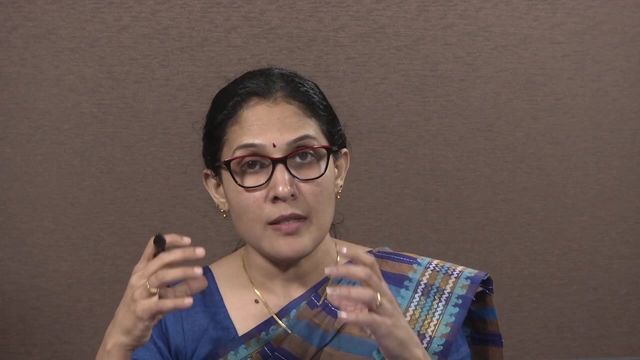 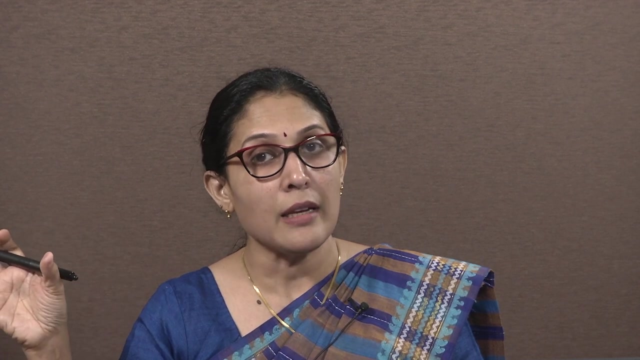 distance is measured. Actually, we will be fixing two points within the reach, within the stable reach, and from one point to other point. How much is the time taken by the float to travel That time? and we already know the distance. both will be noted and if we know the distance travel within that particular interval of time, we can. 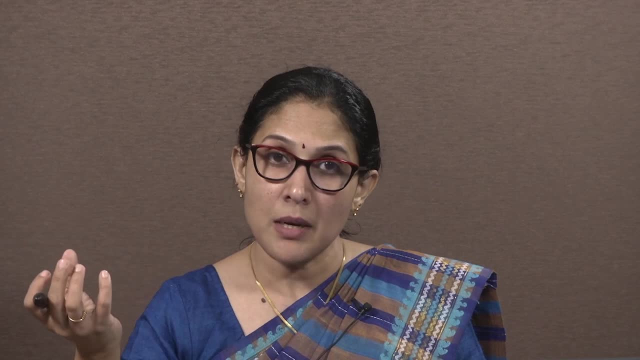 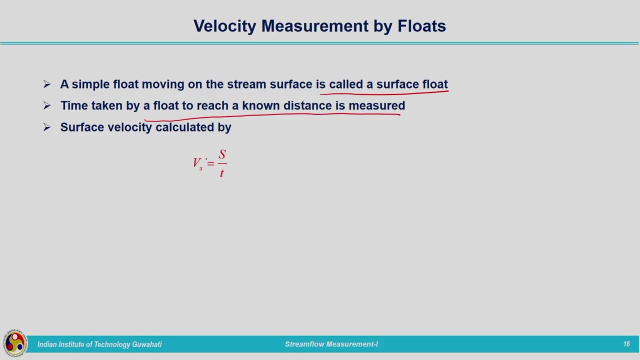 get the velocity with which the float is moving. that is nothing but the velocity of flow, So it can be calculated by Vs. velocity of flow. Vs is given by S divided by T. S is the distance travelled and time is the time interval taken for travelling this much of distance by the float. 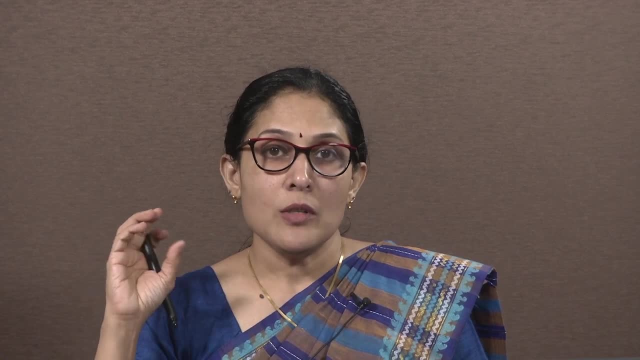 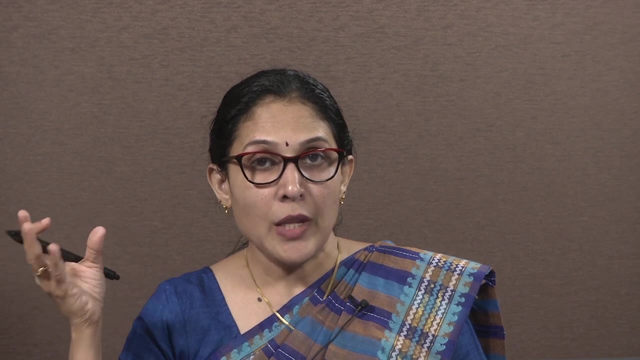 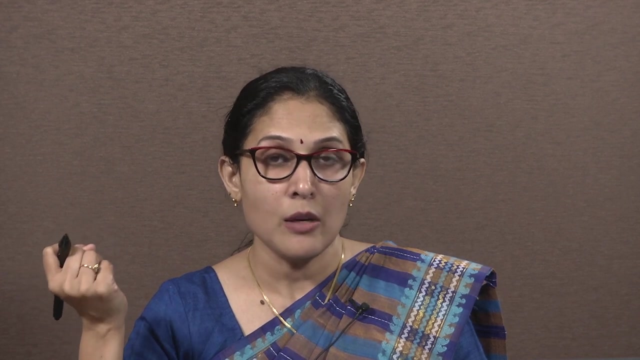 So now it is time to wind up this lecture. So just let me summarize this topic. In this lecture we have seen what are the different components of stream flow. We have seen runoff, base flow, inter flow and the precipitation which is directly falling on the channel of streams. 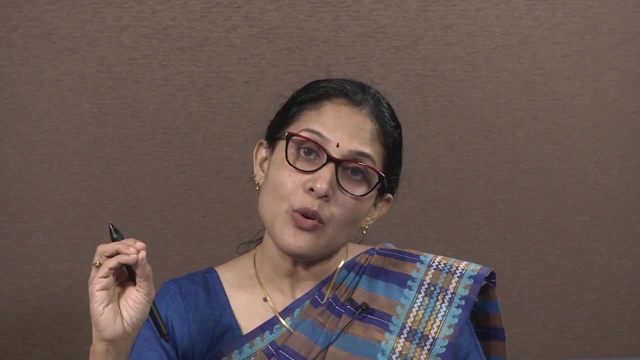 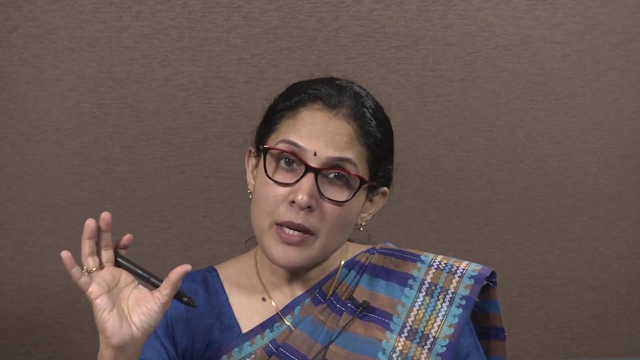 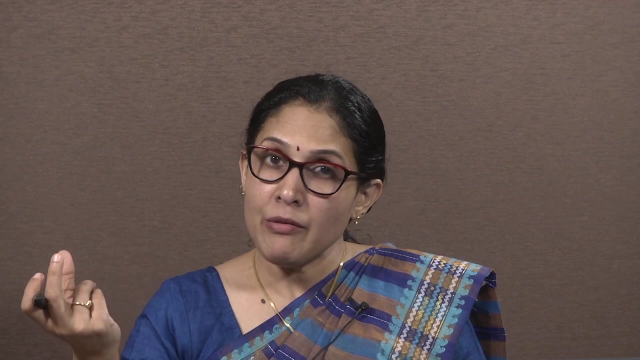 The stream flow values are very important whenever we are talking about the water resources, project implementation and also planning and management. So, how to measure stream flow? Regarding that we were discussing in this lecture Stream flow measurements directly, we will not be doing. We will be measuring the water depth. 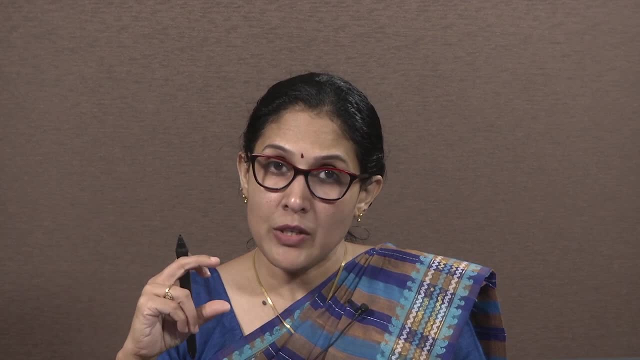 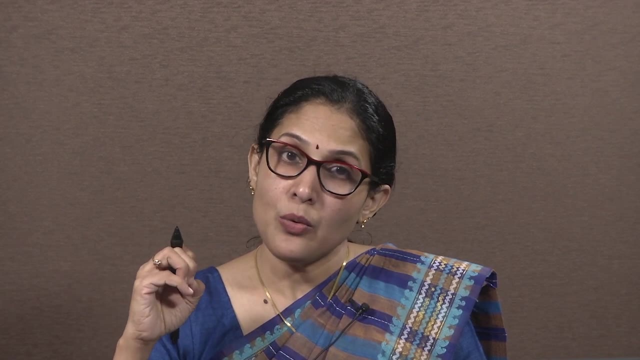 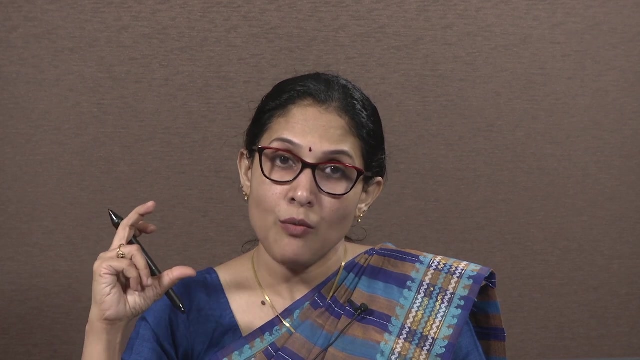 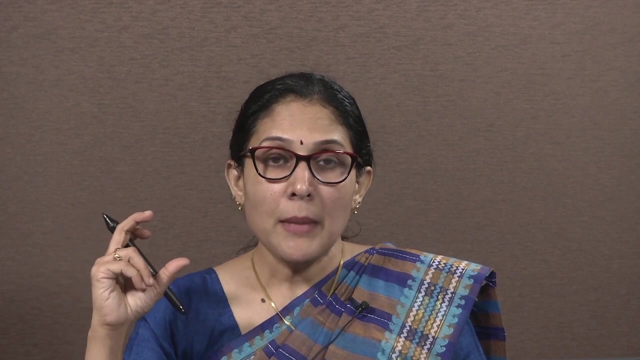 and the corresponding velocities at different points will be measured, and based on that we can calculate the stream flow by making use of the continuity equation. Q is equal to Av, And after that we have seen what are the different ways of measuring stages or the water level in the stream, And also how can we measure the velocity- mainly current meters, which 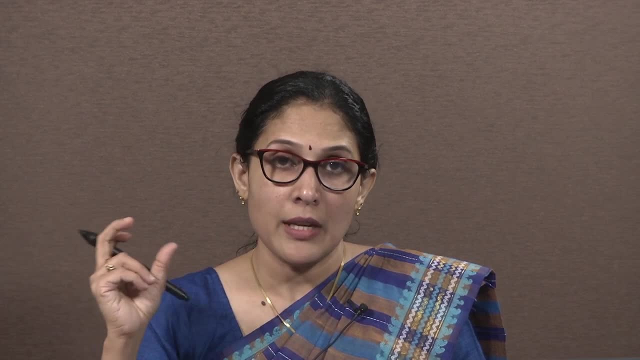 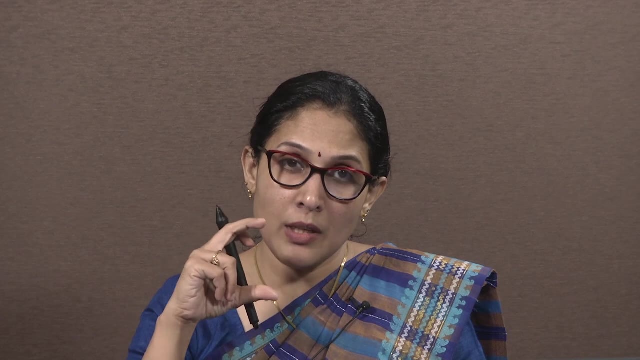 are commonly used for measuring the velocity of flow in a stream and we can get the average velocity at a particular point. So once we know the depth of flow, and also the velocity of flow and the corresponding width of the river also will be measured. So once 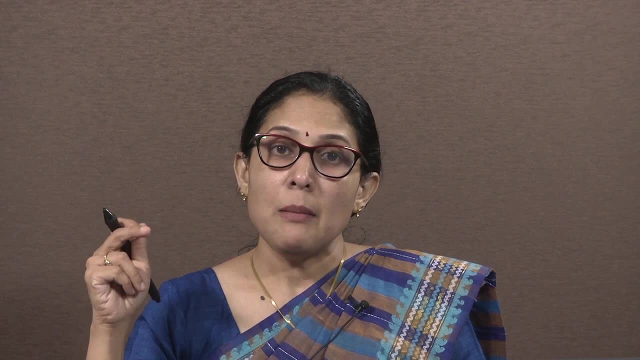 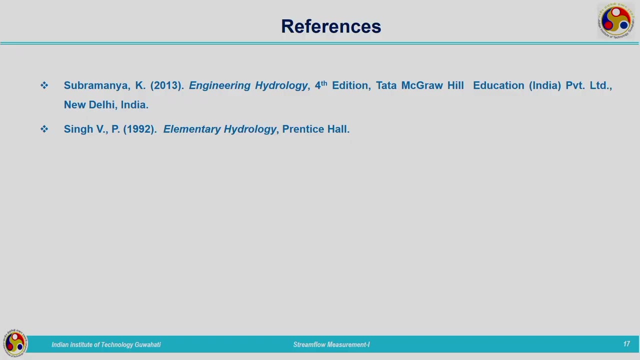 we know, the depth of flow and also the velocity of flow and the corresponding width of the river also will be measured. by making use of the continuity equation we can calculate the stream flow. So, related to this topic, the reference material is Engineering Hydrology by Professor Subramanya. 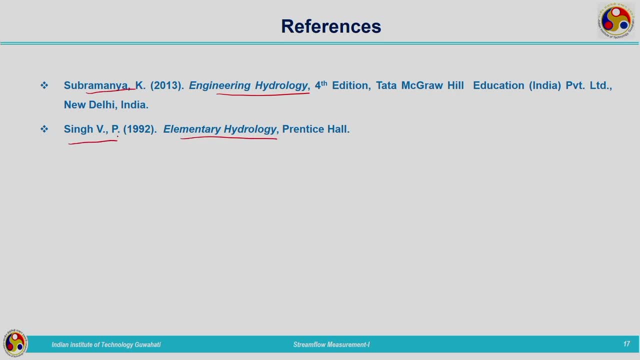 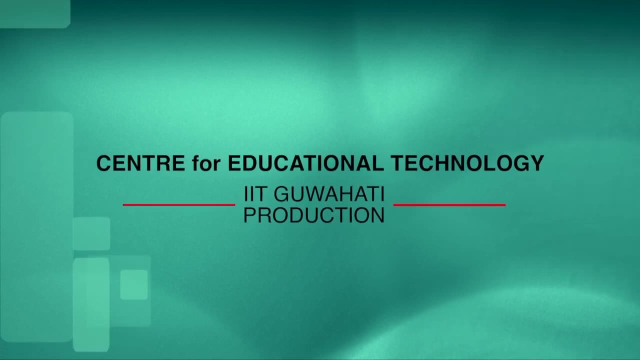 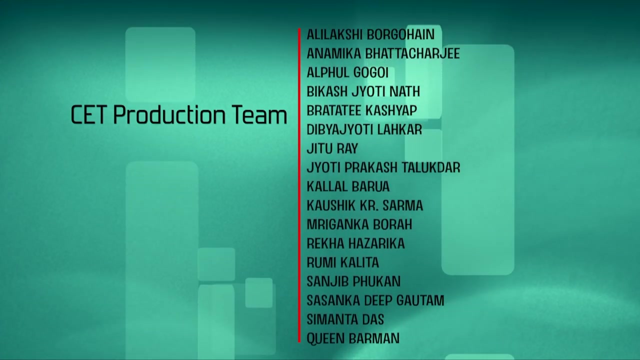 and Elementary Hydrology by Professor V P Singh. So here I am winding up this lecture. Thank you, Thank you.